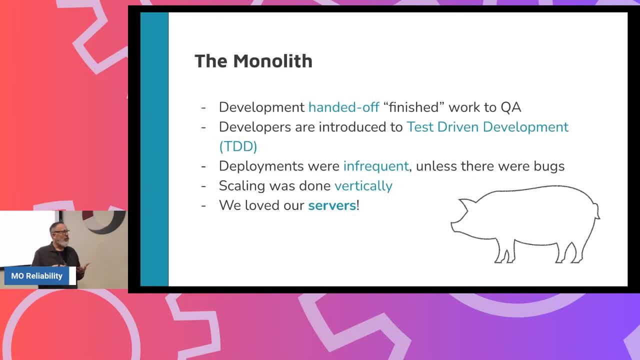 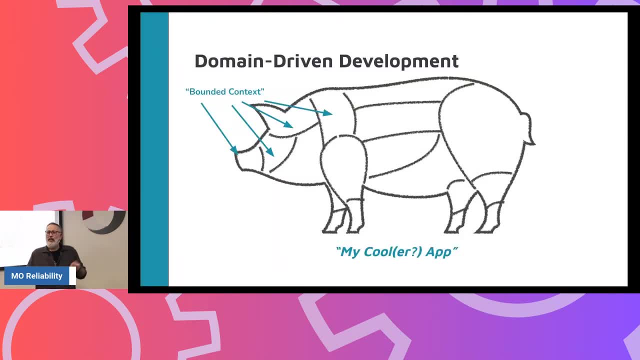 That's when you would do more. Scaling was, of course, vertical, And we loved our servers. They were our pets. Then we kind of started breaking things up a bit. Another familiar image: Yes, Yes, Domain-driven development. We started ‑‑ we realized. 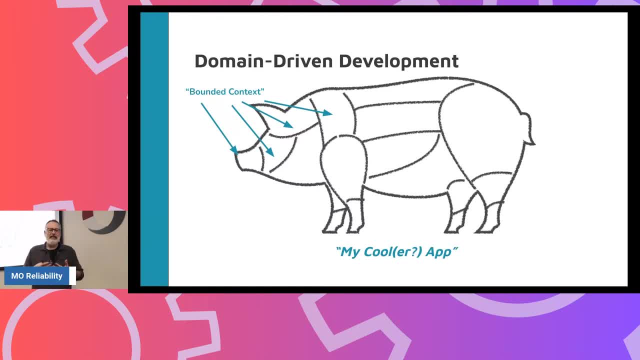 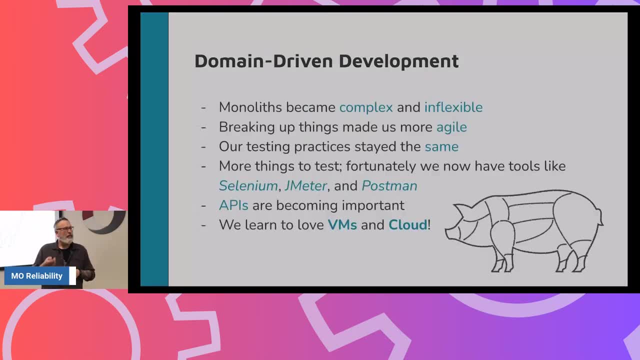 that the monolith is really not the way to go. We started breaking things up based on domain or similar features and that- And that was a cooler app, Right, But yeah, So ‑‑ and really because the monoliths were ‑‑, there's a lot of. 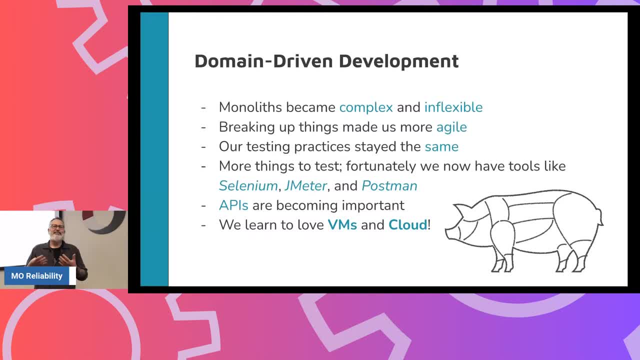 became overly complex and just kind of difficult to work with. i mean, we've had we've had some of those situations here at nisa. you know, breaking up things then made our teams a little bit more agile. they were able to work together in isolation from other teams. 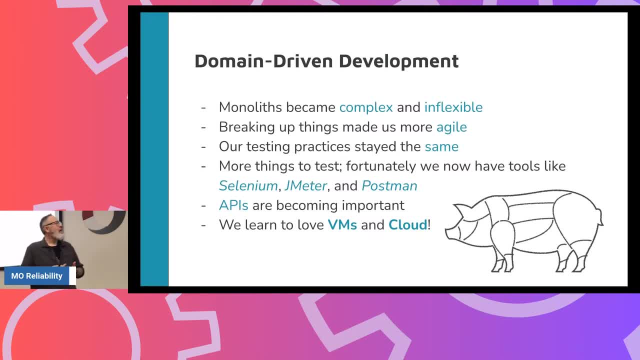 so they were able to, you know, work quickly, or at least more so. testing practices stayed pretty much the same, though. right, we, we created the application, we handed it off, the qa they went through. did the testing? you know, not include? not talking about, uh, you know, j unit we would still. 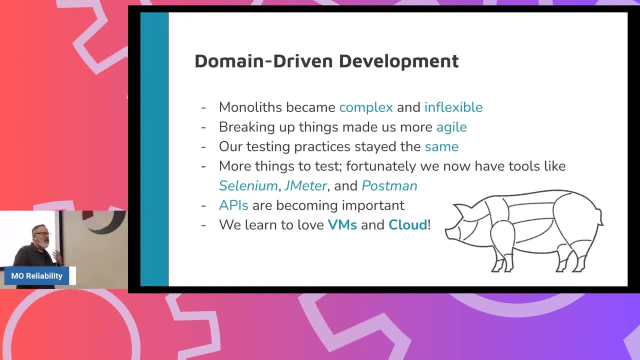 have that in there, the unit tests. but uh, you know, we started getting some more of the testing products. selenium, jmeter, postman, apis were becoming more and more important because now we had these separate deployables and then they would often communicate with each other. so we started. 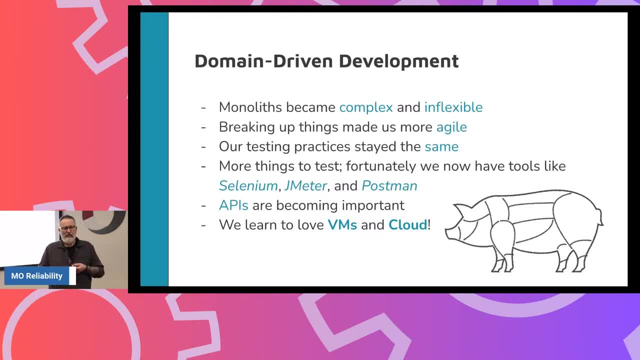 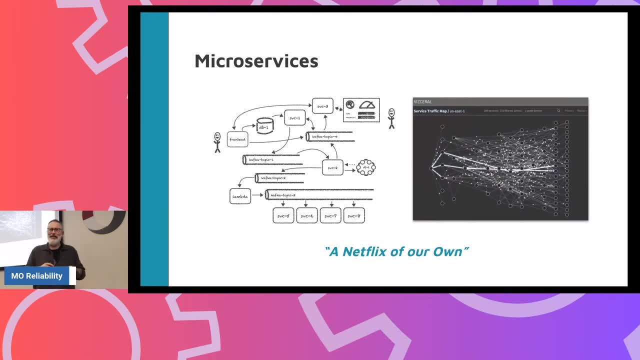 getting into our vms and the cloud at this time. so then here's another one. you might look familiar to you. uh, you know. then we started doing microservices, which was even exploding. it even more right, we were creating the netflix of our own and, of course, the image on the right there. 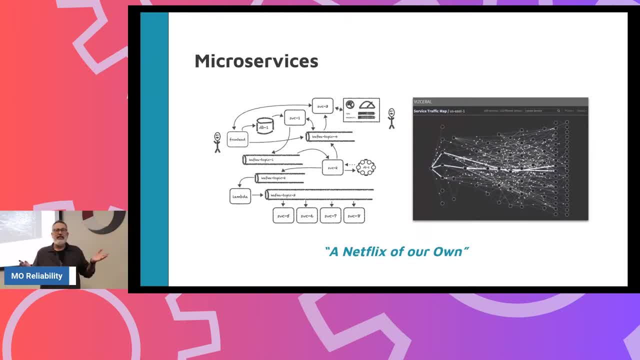 is: uh, is some activity from a netflix service. i'm, you know, sure it's worse by now, but uh, a lot of connectivity, a lot of things interact, interconnecting and talking, and all that so very complicated. you can't really see figure out the whole thing just from one application. 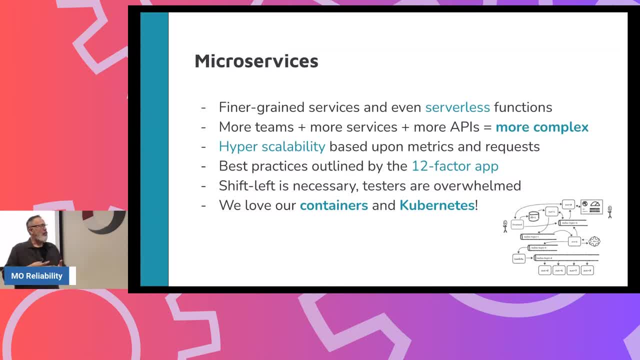 and then the finer grain services were there, so you could even do now serverless functions. so that way then, even smaller, finer grained applications, more teams and services and more apis, the code base. the overall system became more complex. you could start doing some hyper scalability based upon the 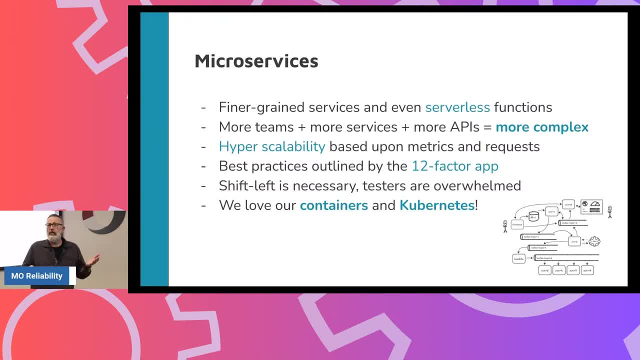 metrics and the request. you know q depth if you were looking at rabbit or kafka, that type of a thing. we started using a lot of the best practices from the 12 factor app, which just made sure that everything was independently deployable and, you know, it encouraged resilience and shift left. 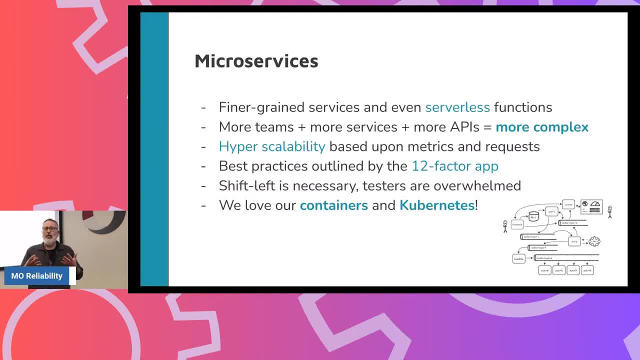 became a thing. that's when we were really putting in a lot of effort to make sure that we were really pushing that. the testers were overwhelmed. right, they're getting this massive services coming through them. they become a bottleneck. developers get upset, so developers need to take on some of 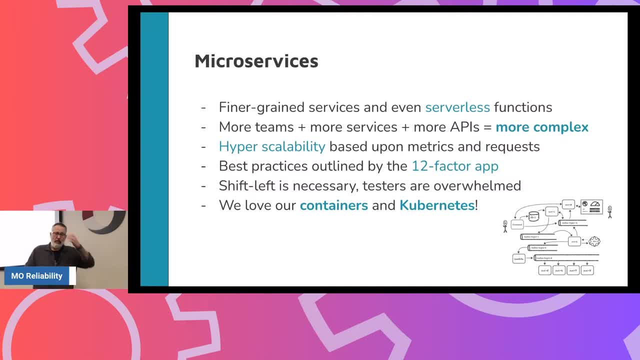 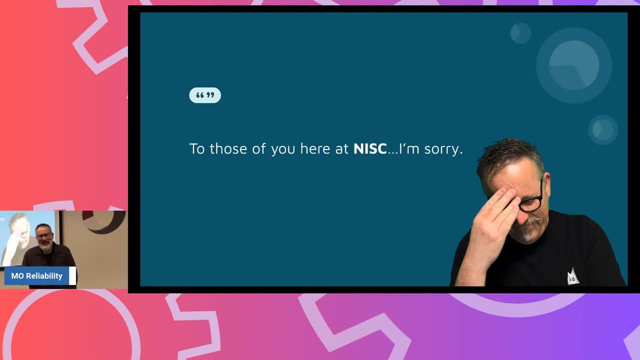 that work and make sure that they're pushing quality before it goes to the testers. and, of course, you know as things evolve- we fell in love with our containers and kubernetes. ultimately- and for those of you here at nisc, i'm sorry- i guess, uh, i don't know- the start of the microservice paradigm here. um, you know it's. 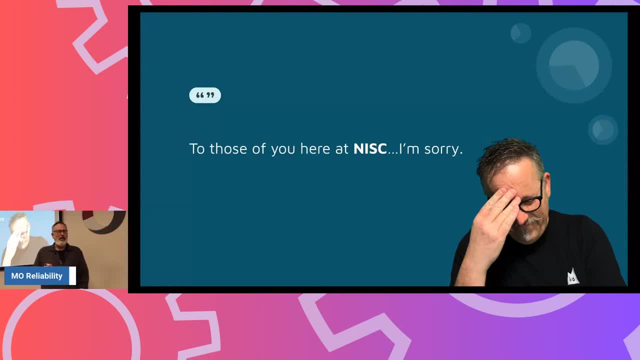 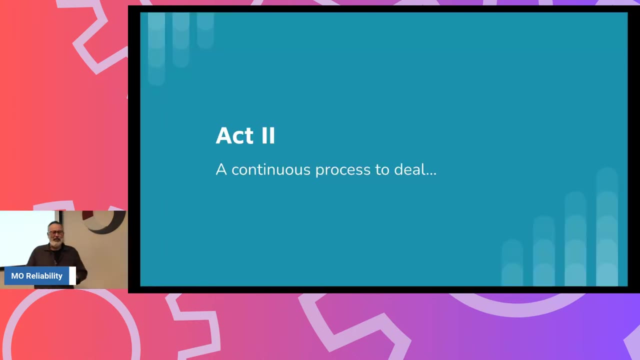 one of those things where it's like: it's a good thing overall, but one of those things where it's like, now that i've come back it's like: oh, maybe we let that pendulum swing a little bit too far and it's uh really causing more problems, but uh, anyway, i digress. so for now, the follow-up act is: 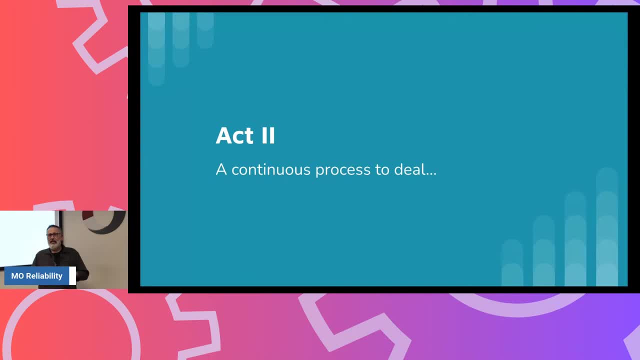 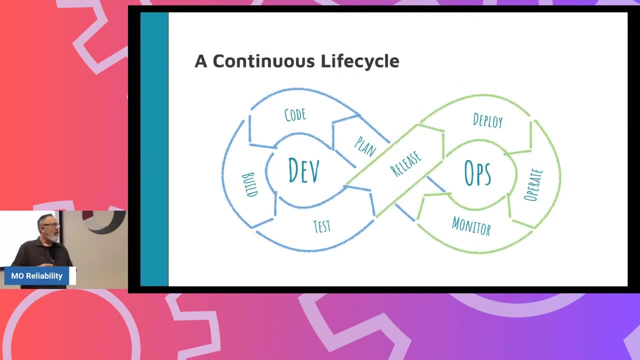 you know the continuous process that, uh, to deal with all these. so here's our actors. we've got the developer, and then we've got the tester, and then we've got our yet another one right code reuse essentially, but uh, yeah, so we have our continuous loop here, our 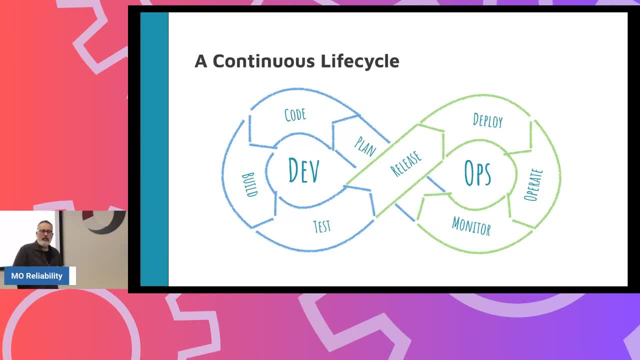 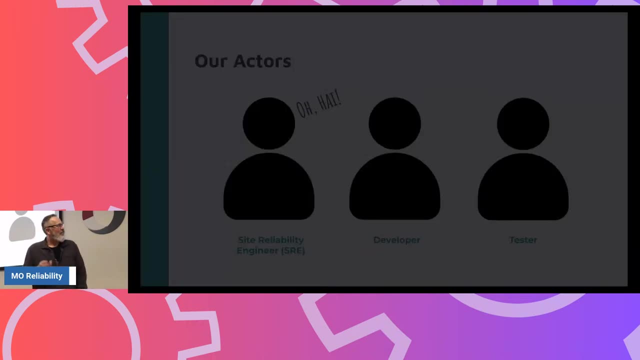 our uh software development life cycle as it goes through. we we created this whole devops uh paradigm and we developed this um uh, the pipeline uh for the testers, and then we had uh. we basically saw that you know we wanted to have a resource for this and i think we've. 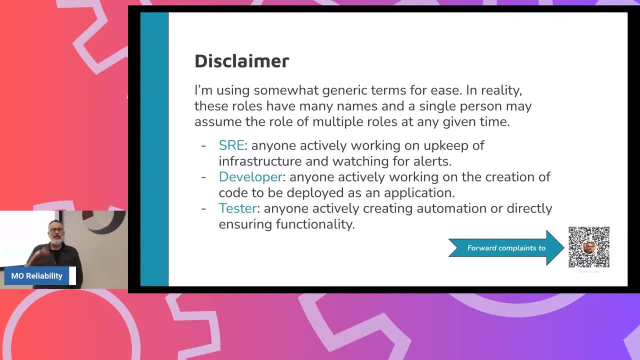 i think it's probably the right time to you know, to really connect with others and with to start working with other stores and with other companies- um, you know all the different loving ones who have been working with us for, you know, the last couple years, basically our 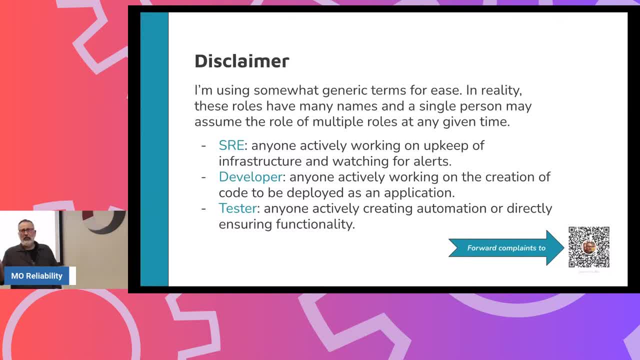 third year now has been really successful, and i think the reason for this is because, in fact, we've been working with them a lot, too many years, and we've had a couple of cases where they've been working with a few companies for some time and then we've come back and we've worked with a lot of 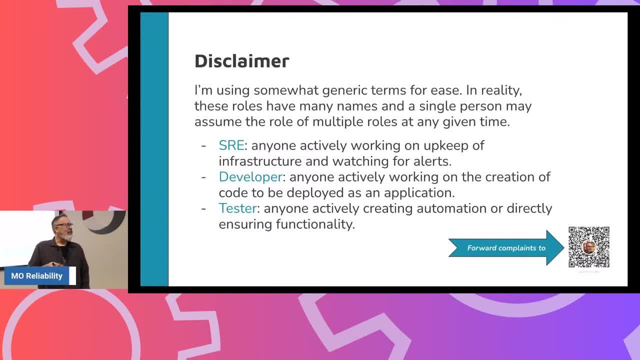 and all that to platform engineers, things like that. Developers are, you know, creating applications, features for consumers to use, And then the testers are just anyone involved with ensuring the functionality, And then, of course, you're going to be wearing multiple 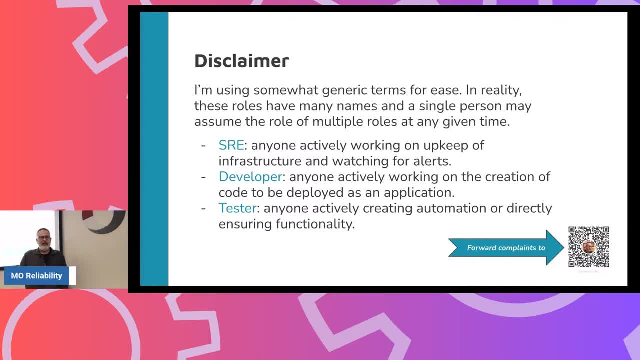 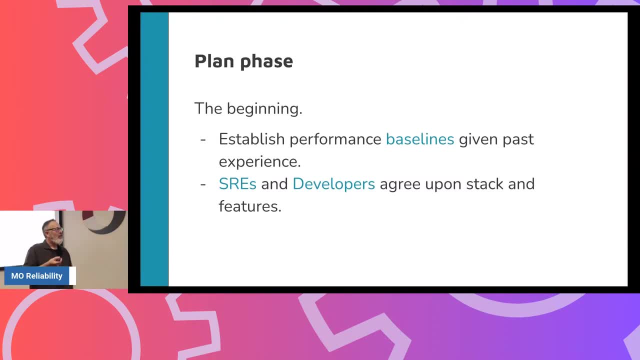 hats. You know, it just depends on what you happen to be working on at that time. So here we go. So let's start at the beginning, right with the planning phase. So with the planning phase, you know, we want to establish really baselines for the performance Bless. 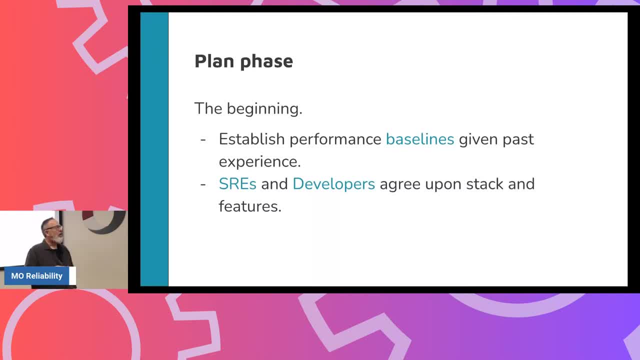 you. You know the SREs and developers can agree upon the stack and the features. You know you can't really go and say: developers, you know, get the next shiny thing. They love that, It might be the next shiny thing And I know I'm one of those that fell into that. 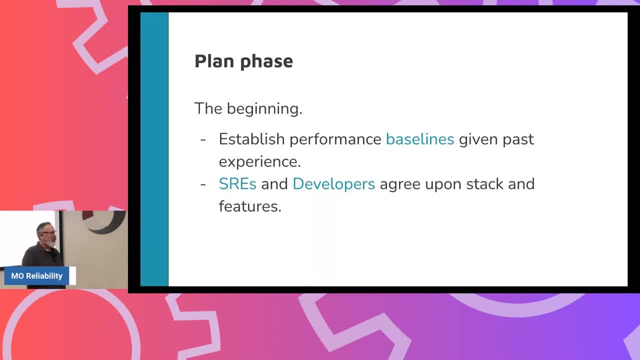 trap as well. right, I like shiny, But it's one of those things where you have to agree upon it, because The SREs are technically the ones that are going to keep the lights on and keep it operating right, So they need to be able to have that depth of skill and knowledge. So you can't. 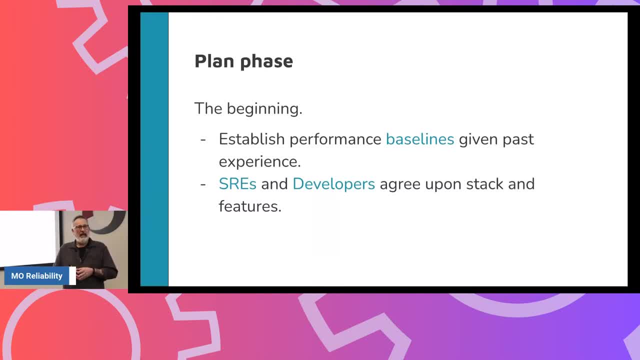 just keep getting the next new shiny thing, because then you're not going to have that depth of knowledge. T-shape right, You want you know, wide breadth of skill, But then you want to be able to have a deep you know ability and knowledge. 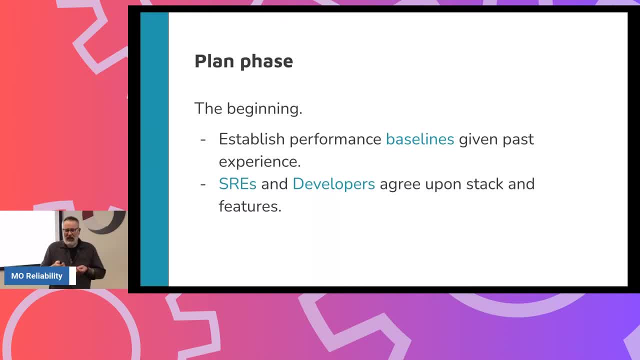 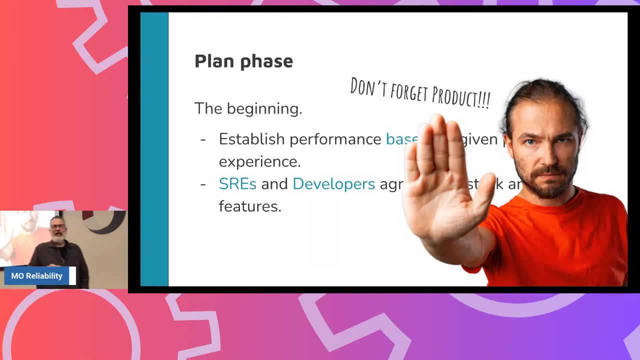 Okay, And at least something. It can't be just all shallow and going wide, But yeah, But we forgot the product. We got to let the product folks in there. They're going to have their comments there about what features that the SREs and developers are going to plan to work on. So 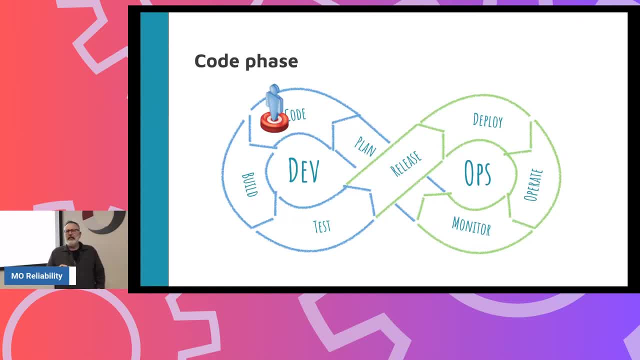 Next, we move into the code phase Now, and this is one of those things too, is that? obviously, with this diagram, everything seems like it's sequential right? One phase, then another, And then we move into the code phase Now, and this is one of those things too, is that? 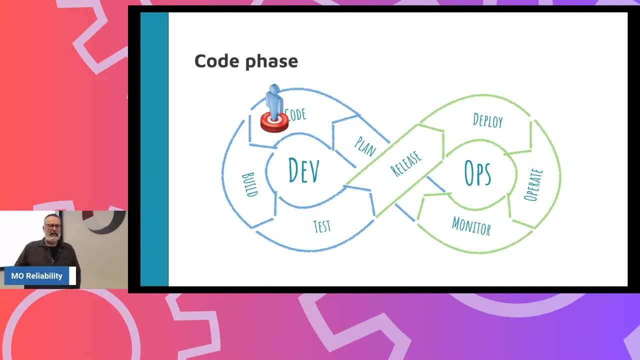 obviously, with this diagram, everything seems like it's sequential right, One phase then another, So it's one phase, then the next phase and then the next, And it's never like that. We all know that from daily operations right, These are going to be going on at the 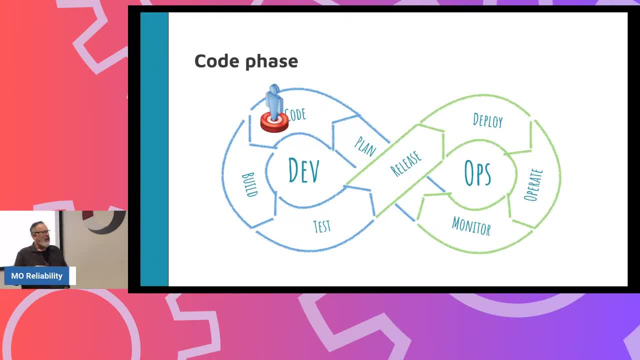 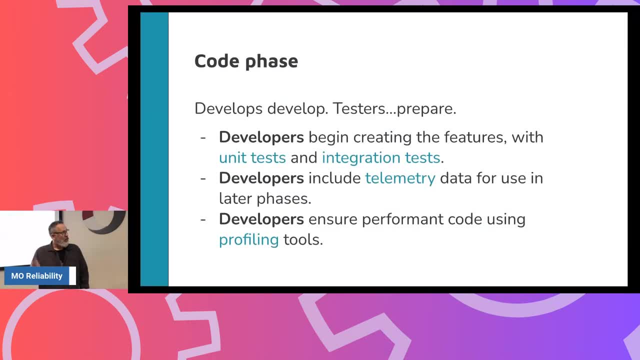 same time overlapping a bit all that good stuff, But for purposes of this talk, we'll just keep going with this. So the coding phase. Now, here's where the developers are really doing their thing. They're creating the features, They're bringing in unit tests, They're using. 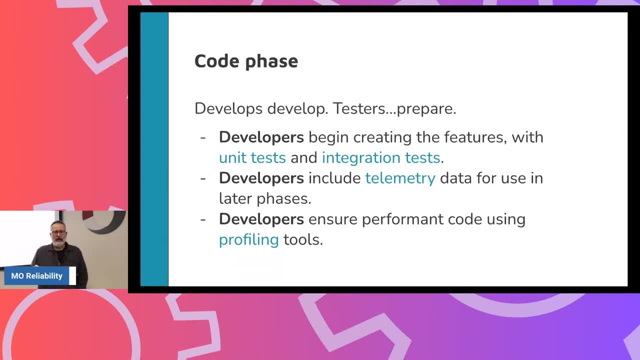 like test containers to be able to do integration testing. you know shifting left again. you know making sure they include telemetry, because once this, this application or feature that they're working on, goes past them, the people that are operating the software need to be able to have visibility. now the 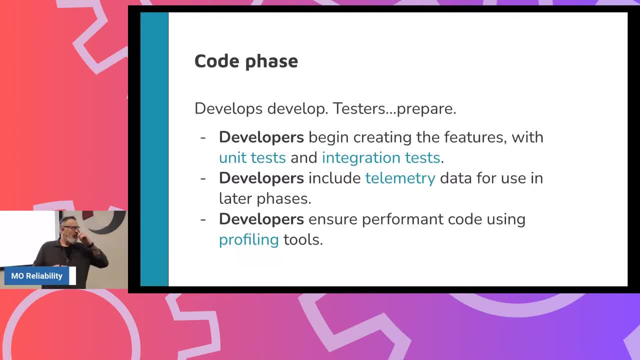 telemetry data is how they're going to be able to do that, so they need to make sure that they're including that they can use. you know different technologies as well that don't have to be coded in, but this is probably the the better method you know, and then again developers are ensuring the performant. 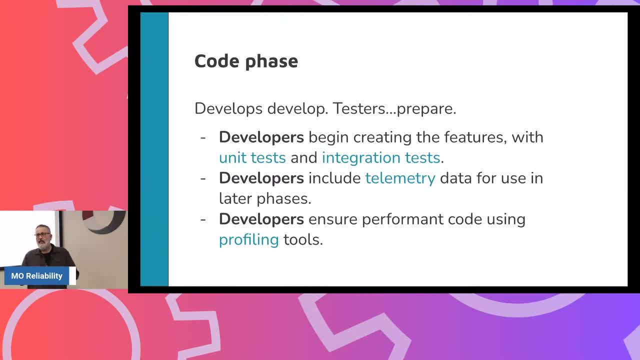 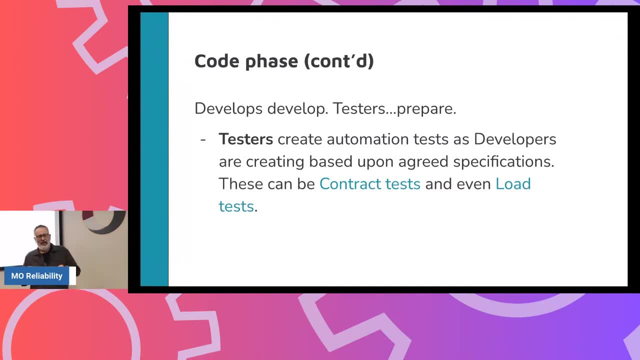 code by profiling. they need to do profiling before it goes beyond them now with the code. oh yeah, so code phase continued. but yeah, so the testers should be creating their automated tests. you know, against what the developers are producing and based on, like the things like contract tests and the load test. they 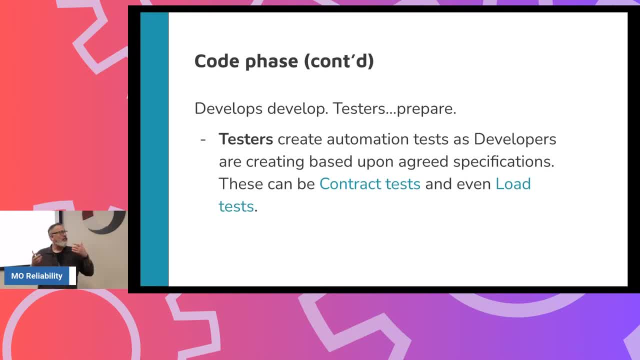 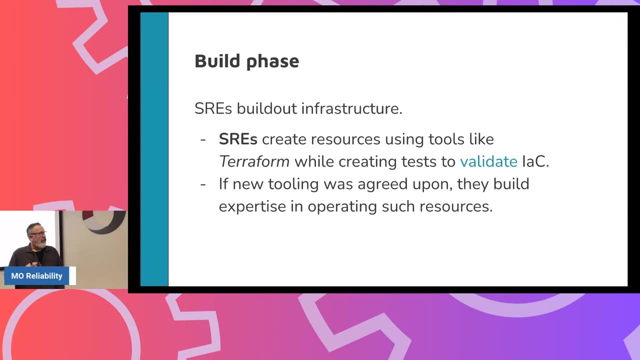 can start getting that prepared. you know, obviously they're not going to be running the big load tests as they're developing- because it's probably not ready yet- the software from the developers, but preparation so as we move into the build phase we've got the SREs building out the infrastructure. this is 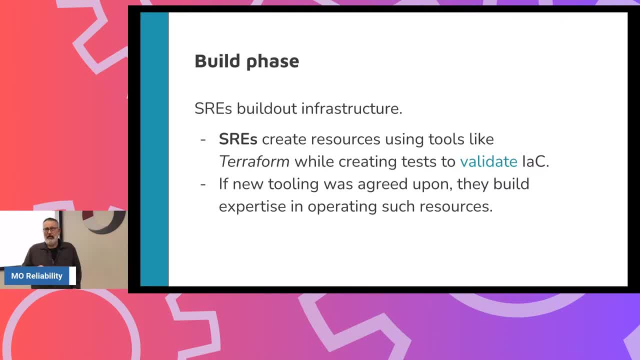 where they're going to be doing things like. you know all the good fun with Terraform right and building out that, all those resources in the cloud- you know AWS or GCP and all that- but the important thing is that testing on there, they need to also make sure that their 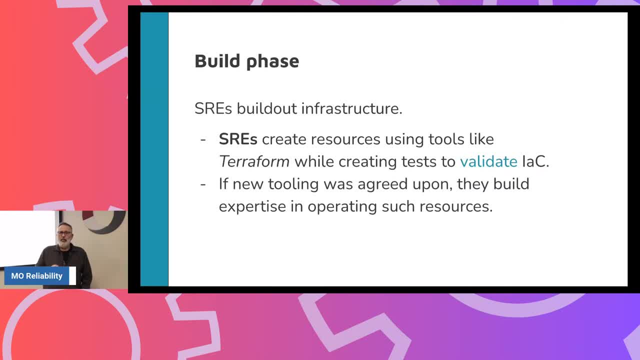 infrastructure, is code works correct, you know, and in that there's no confusion or you know unknowns about when the next one gets applied. what's going to happen? you know, is it going to be destructive or is it gonna lose focus? and you know, that's all. it depends a lot here on this part of the level. 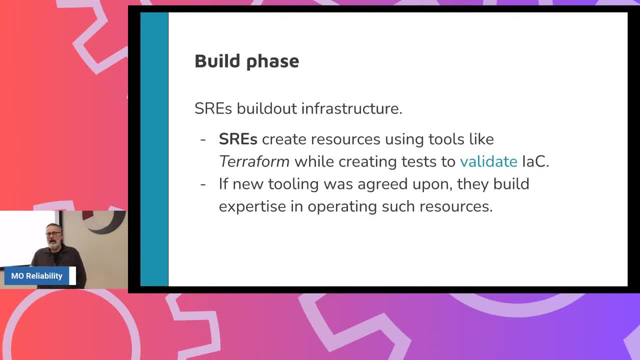 data or things like that. This is all things that we've got going on here at NISC. you know we've got the testing framework in there and then, oh yeah, so kudos to you guys for that. And then again, yeah, if the new tooling was agreed upon- you know that shiny new. 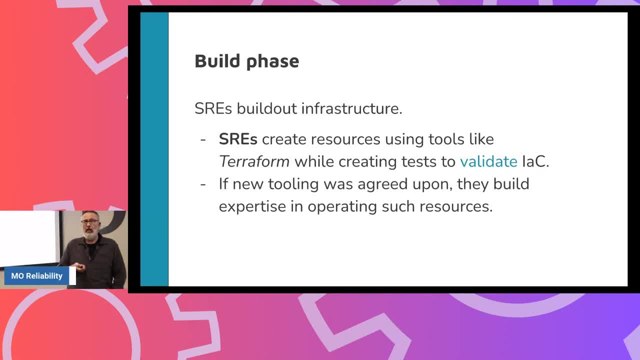 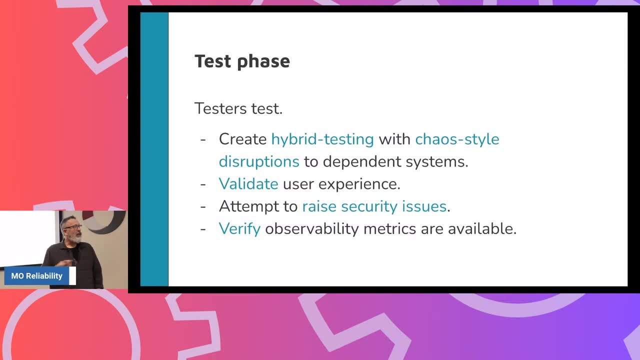 tool. this is the point when they should be ramping up on picking up on that knowledge. Okay, the test phase. so again, you know this is going to be going on at the same time as things are being produced, But, yeah, testers can do hybrid testing and then with chaos. 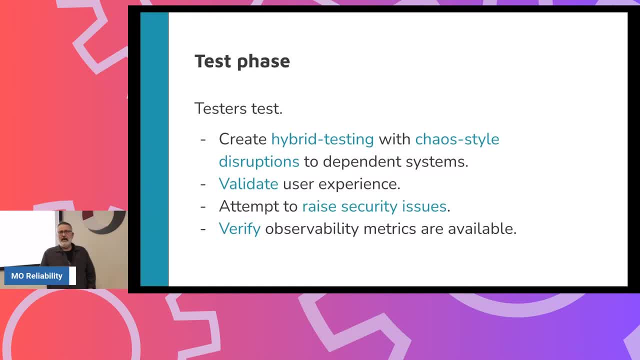 style disruption, So the hybrid testing, meaning like, if it's a user interface based, so web application. they can use tools like K6 with the browser extension that can actually replicate a user Actually clicking on the site and you can do things with the back end where you take. 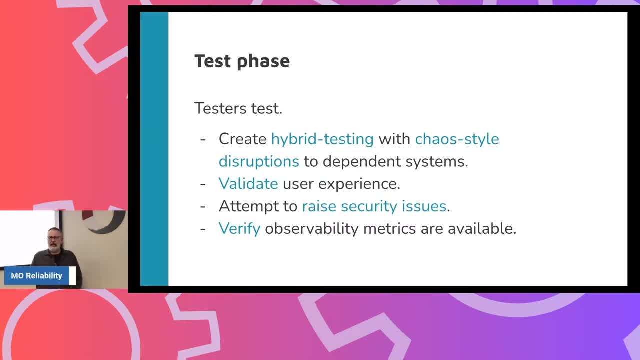 down the service, or you inject latency, those chaos style experiments, where then you can see how the front end is actually affected by those outages or slowdowns you know, just to validate the user experience. And then, here too, you know, raising security. 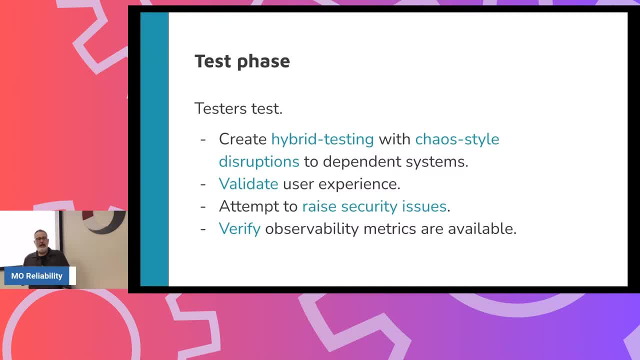 issues if they can, if they have that knowledge to try to figure out if there's ways to get around that. So you know we're going to be looking around some of the precautions that are in the code. You know your SQL injection type attacks or you know, potentially even denial of service. 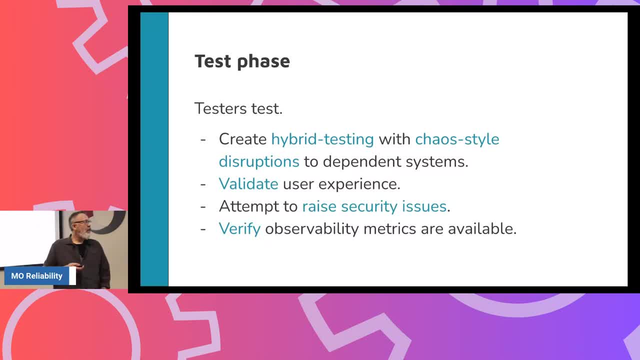 But denial of service is probably at a later point, But try to, you know, find it early And also, too, make sure that the observability data, that's in the application that the developer has coded in, are actually producing things that are valid and are, you know, maybe if 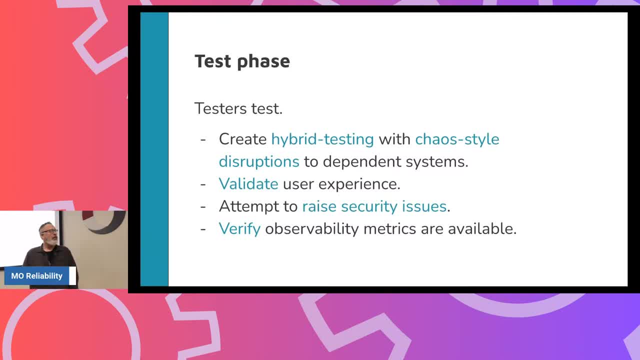 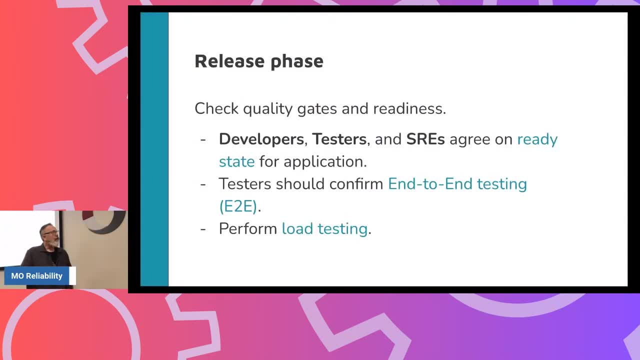 the developers are creating dashboards and things like that that you know, make sure that those are good. So then we had the release phase, which you know the developers, testers, SREs- you know everybody's agreed: We're ready to go. This is past our quality. you know requirements. 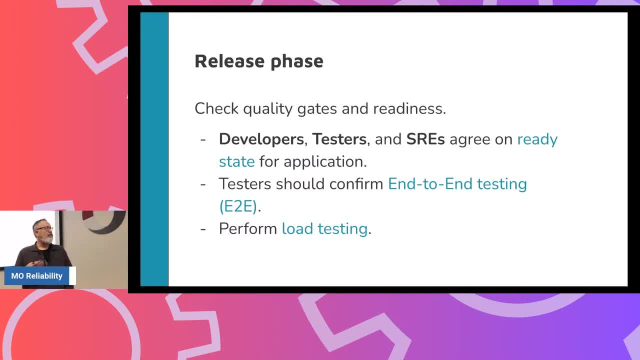 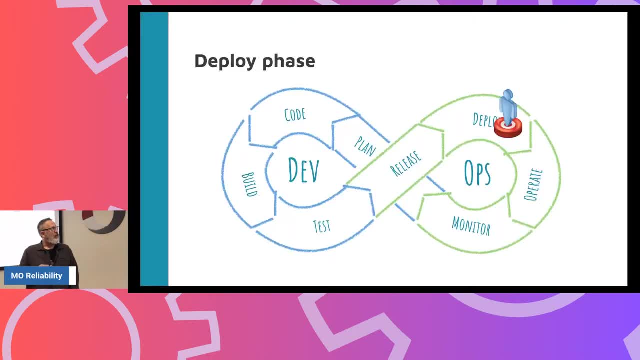 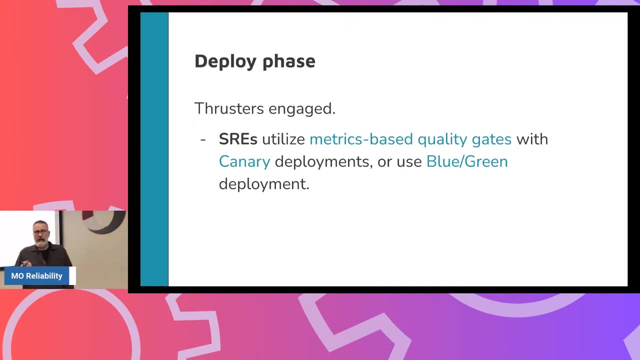 You know this is when end-to-end testing should have been completed. you know, load testing, the real load tests, Right, Just making sure that that's all done. And then if we go into the deploy phase, you know quality gates. 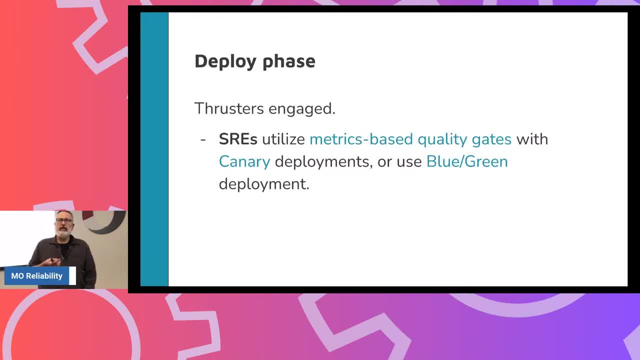 So there's projects like Keptin which can be running in Kubernetes and it'll actually look at your Prometheus metrics as you're doing a deploy. It actually kind of controls the deployment And then that way then it can tell if oh. 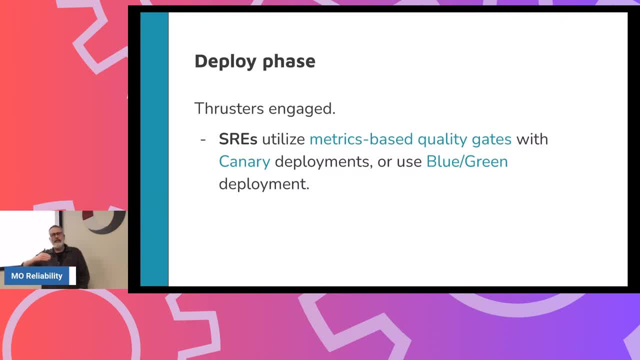 okay, this canary version is coming out. We're seeing a difference in the you know, Prometheus or whatever metrics that shows like we're having a slowdown, So they shouldn't proceed. So it can do some quality gates in that manner. 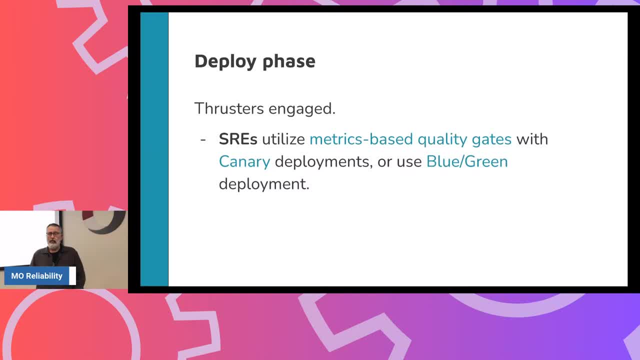 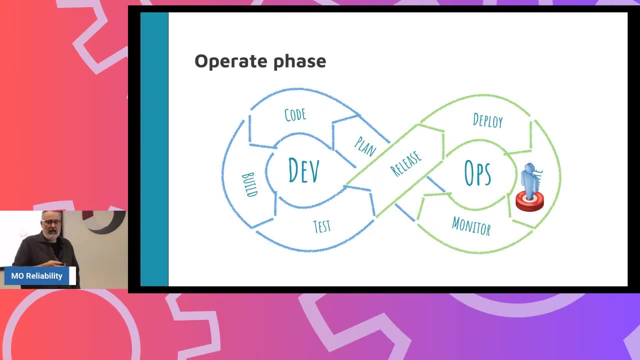 And then also with, of course, the canary deployments and blue-green. So, having that all ready to go and then test it And moving into the operate phase, So here's where the SREs are living most frequently. Okay, Most of the time, right. 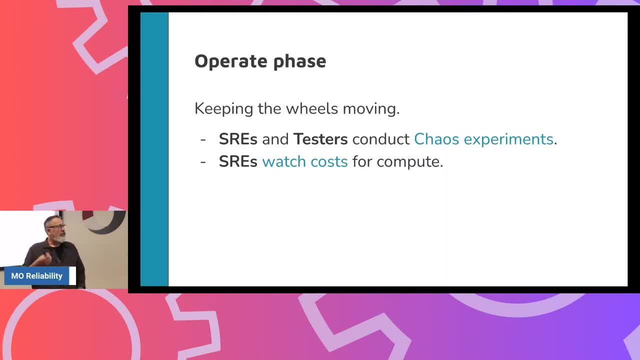 This and then the next we'll talk about. But you know, this is where, in a mature environment, you can do chaos, experiments against your production. But yeah, you can have your- you know your- testing days or play days or whatever, and 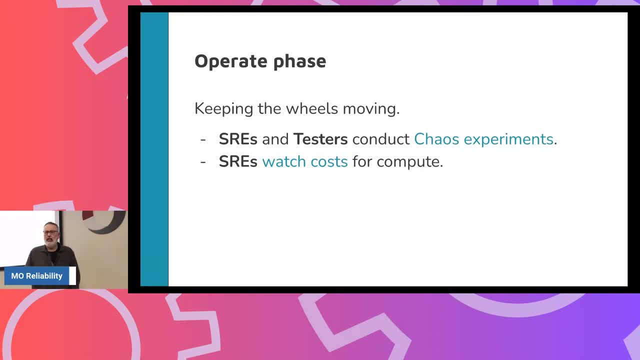 then do some experimentation like that, you know, in a controlled manner. You don't want to take down your production system completely, You just want to find its faults, You know. so take it to the edge where you know it's going to tip over already from earlier. 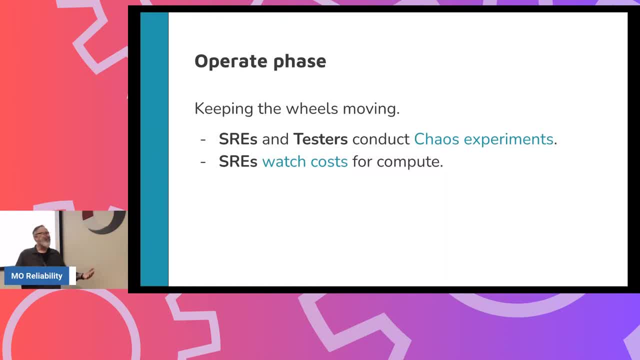 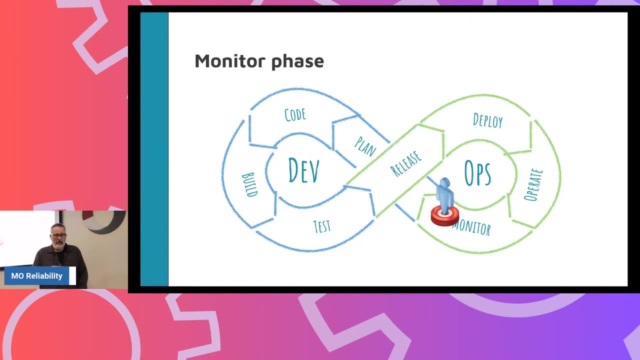 testing in this life cycle. you know, But yeah, but don't try to break things completely And then keep an eye out on cost. This is where we can start doing the FinOps type things, But let's see Okay. 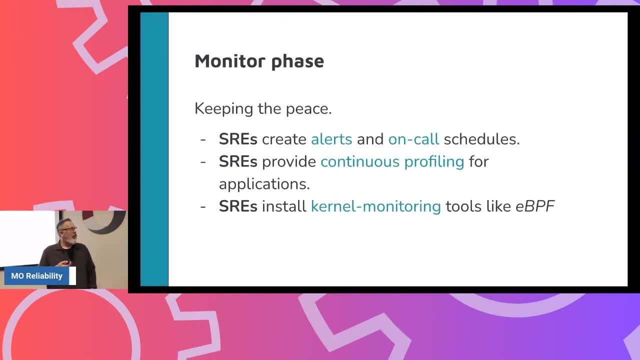 And the monitoring phase, which, of course, is the SREs again creating their alerts, maintaining the on-call schedules- Okay, Watching continuous profiling, holding developers' feet to the fire, if there's a second-level issue that they need to look into. 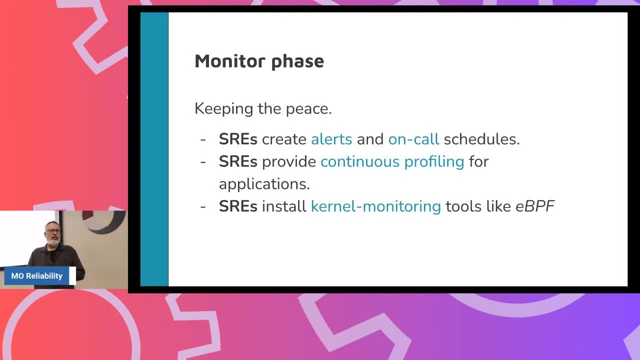 You know they're going to maintain who is the owner of certain applications. you know, and then yeah, who to contact if it needs to go to the next level of support, Because, again, we can't expect the SREs to be the subject matter experts on every. 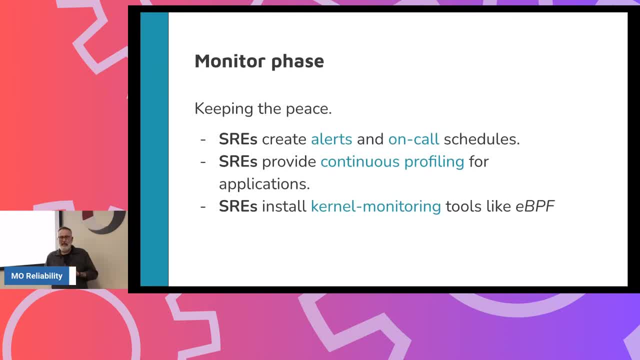 single application, every single service. It's never going to happen. But they need to know, they have to have that call tree type thing of who to get who to call for the issues you know. And then this is where we can include the kernel-level monitoring with tools like EVPF. 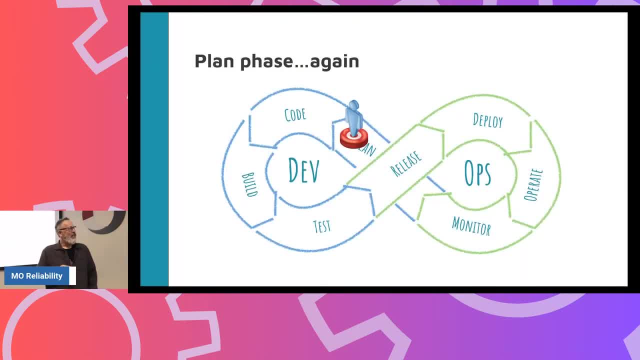 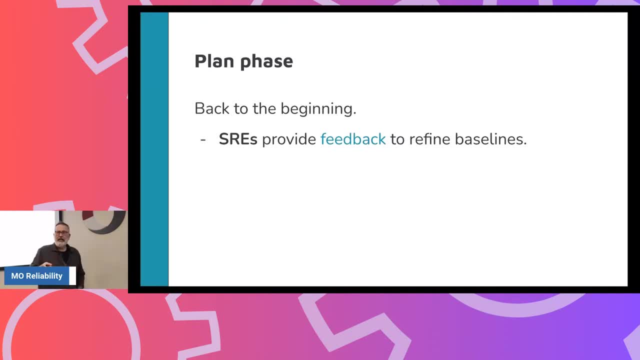 you know, CILIUM, yeah, And then we proceed back to the plan phase. So this is where, then, how the SREs- they need to give the feedback back to the SREs So that they know what the issues are, you know. 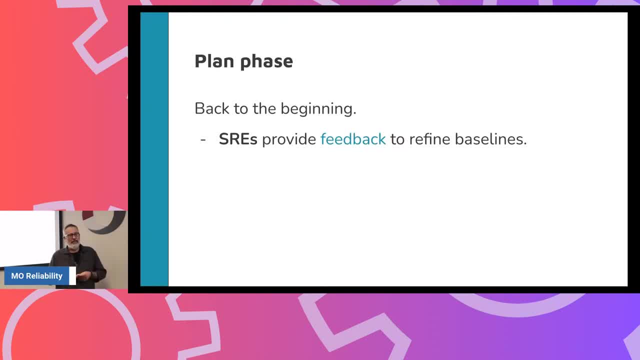 The developers can't fix it if they don't know what the issues are. You know, developers shouldn't be completely, you know, ignorant of what's going on with the production code that's running, But they're focused on the features, right. 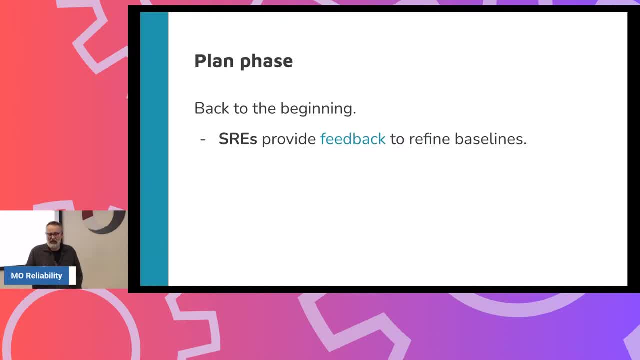 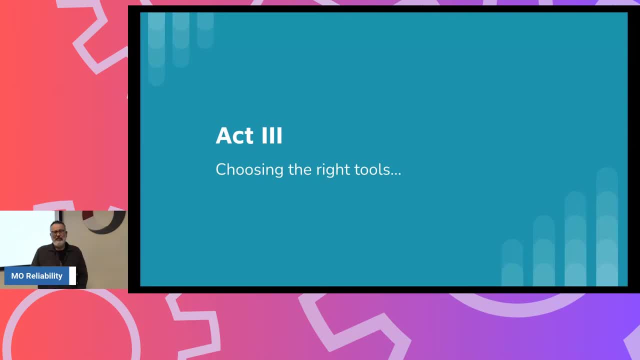 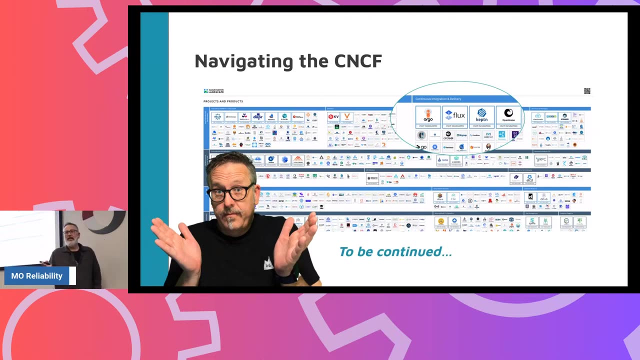 So they're not going to be paying as much attention. So they need to know, They need to get that feedback. All right, Thank you, All right. And then now there's tons of tools. So yeah, there's, I don't know, I'm not going to tell you which ones to use. 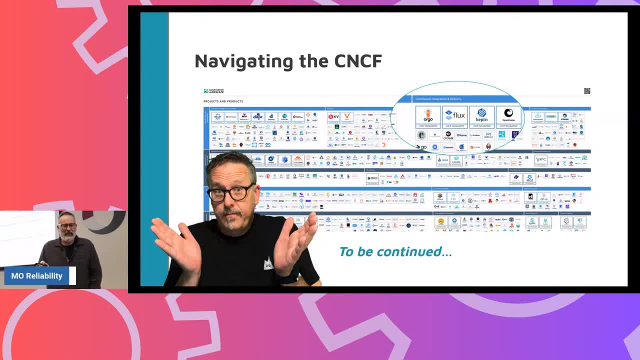 I don't know right And every situation is going to be different. The CNCF has loads and loads and loads of different products that need to be evaluated and potentially used to solve the issue, But you know that's going to take ways. 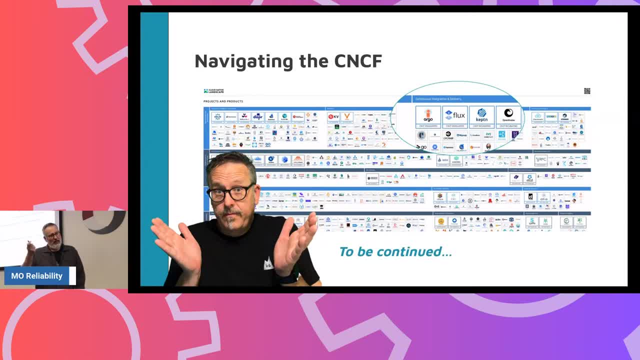 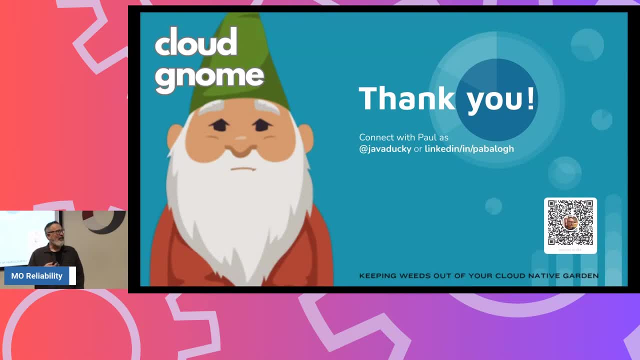 It's going to take way too long to try to go over, And, although I do have plenty of extra time, I thought for sure this was going to be very long. But yeah, So that's, I had to leave it there. 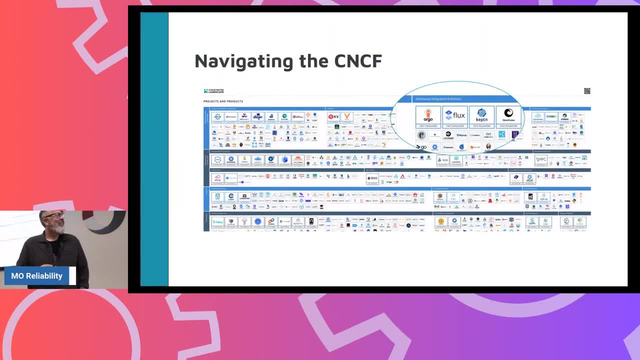 So questions: Yes, Can you talk more about chaos engineering techniques? Well, I can tell you from like. so with K6.. I used to work for Grafana and K6 was one of their products. So yeah, So we did do some chaos experimentation. 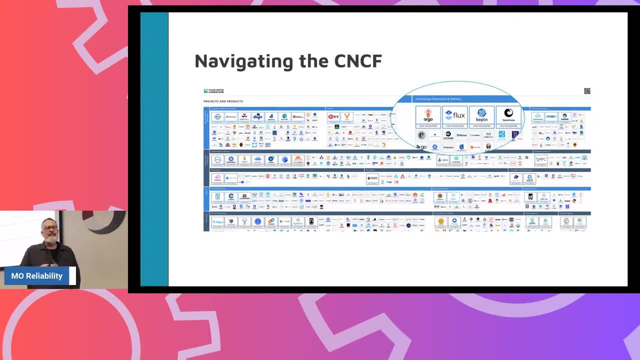 So you could actually do things like we were doing, things like you know, injecting latency So you can play around with your network connections. You can make it where it's like: okay, maybe 50% of your calls take, you know, 10 seconds. 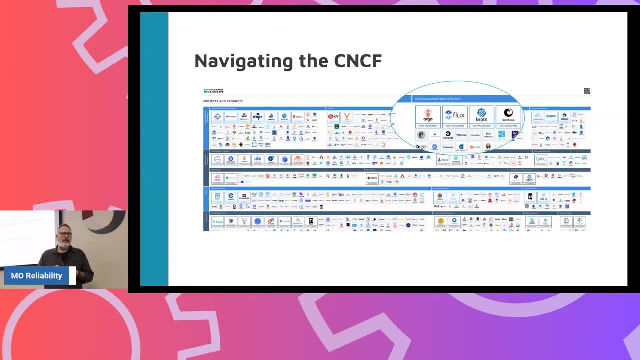 additional What happens, You know, or you can sit there and you can kind of test Kubernetes, And then you can kill people And you can kill pods. You can target pods or services and bring them down and just see how the rest of the application works. But yeah, I mean, that's pretty much most of that engineering It's- you can really get your most of your chaos. testing is down to latency and then exceptions. You can simulate exceptions bubbling up from a service as well. 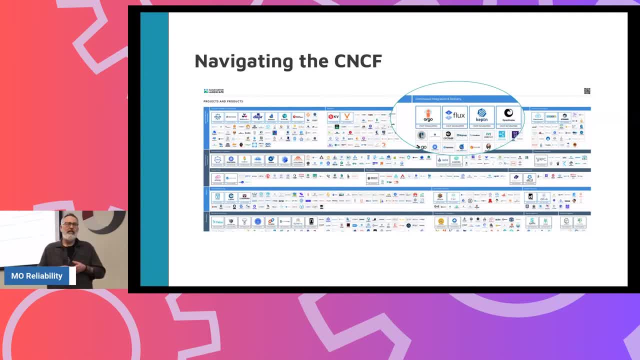 I thought they did more, with entire microservices being down, for example. Thank you, Yeah, Yeah, Yeah, Yeah, Yeah, Yeah. Hello, Yeah, Uh-huh, Uh-huh, Obviously Uh-huh, Yes, Uh-huh. 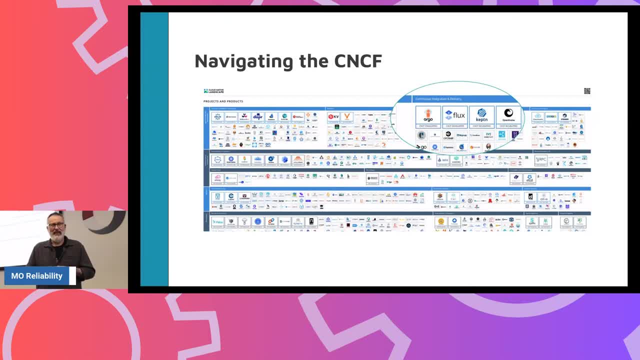 Okay, Sounds good. Yeah, I mean, you could do that. So the chaos testing that we did with K6 was pretty much again, like I said, the services and deployments, or pods rather, and then the latency. But yeah, you could do things where, like I don't know, maybe you're rolling back a. version or something from a service To see how things behave. So then that way, then if you do have API issues, but API issues should have already been caught with contract testing earlier in your phases. But yeah, I think for us, all of the chaos, testing started with just trying to restart our Kubernetes. 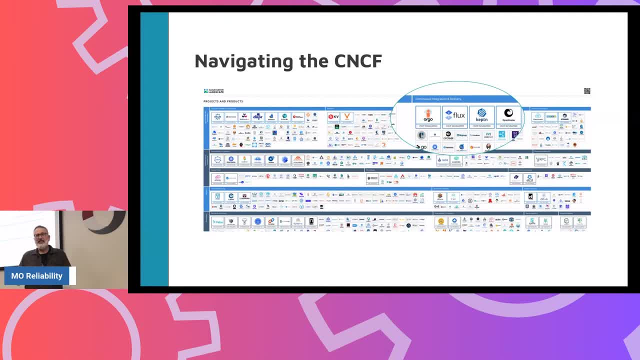 workers. Yeah, That alone was enough. chaos, Everything trying to yeah, everything trying to start up, and then one service not being there. that's core and yeah, Yeah, Yeah. But that's just the maturity level of the organization and frameworks. Yeah, And that at least is something that you know Kubernetes does kind of take care of, where it'll keep killing the pod. But yeah, it might cause all kinds of havoc on your system overall while that's happening. But eventually it'll get consistent and it's going to try anyway. 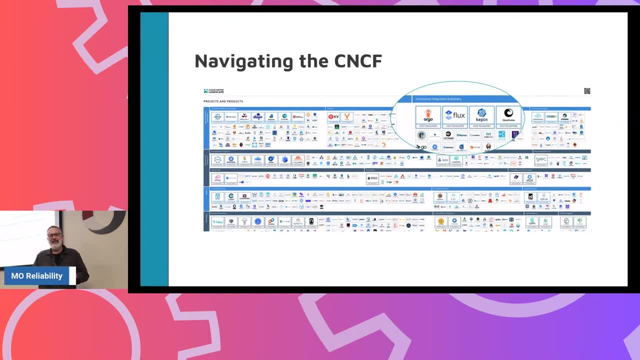 Not consistent, but you know to what your state is your desired state. Yeah, All right, Yeah, Yeah, Thank you, Thank you. Okay, I think we're ready to go. All right, Yeah, Yeah, All right. 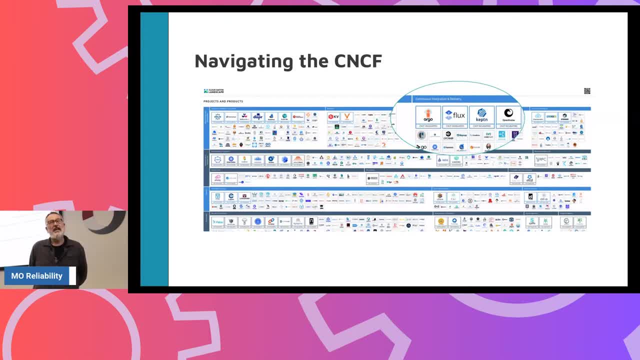 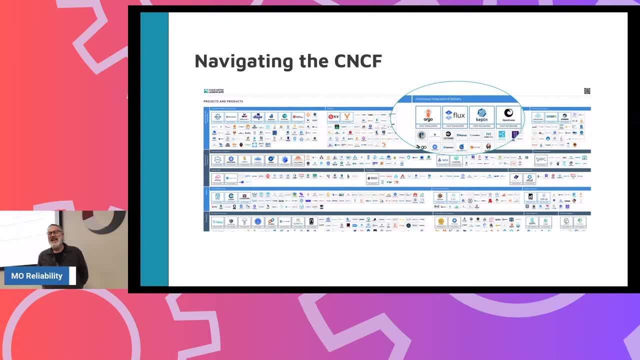 DNS, it's always DNS, right. It's something that is so central and key to everything that, yeah, DNS fails, then basically everything right, Caching, and yeah, yeah, Yeah. So you said you weren't going to present any paradigms or tools. 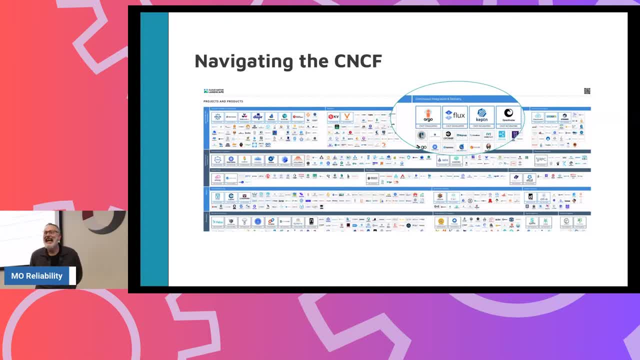 that you were going to recommend, but if you were just a little bit, Yeah, let's get to that. Is there anything on the map there? Right, Yeah, no? So yeah, the question was to repeat. the question was: 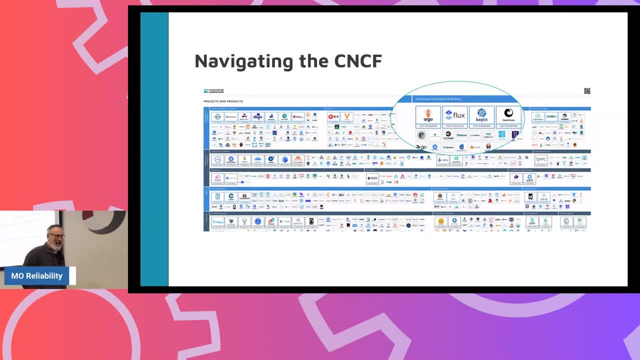 is there. even though I said I wasn't going to recommend any products or paradigms, is there anything that I would really recommend? that's on the CNCF landscape And, to be honest, even though, as an investor, there are so many projects there that creep up. 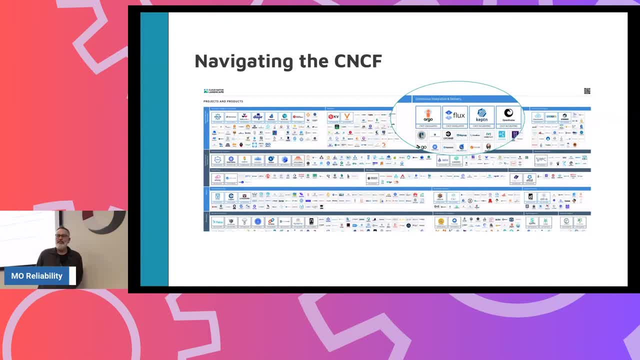 and you just don't know that they're there. You know, because you just haven't heard of them, because there's just so many, It gets lost in the noise. Yeah, I don't know, There's so many of them. 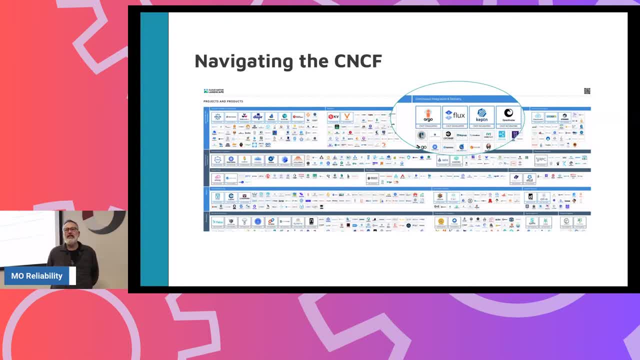 And that's why it's like, yeah, there's no way we could really go over this. But my hope is that if there's a specific interest in a certain aspect, you know I can do some digging in a little bit more research. 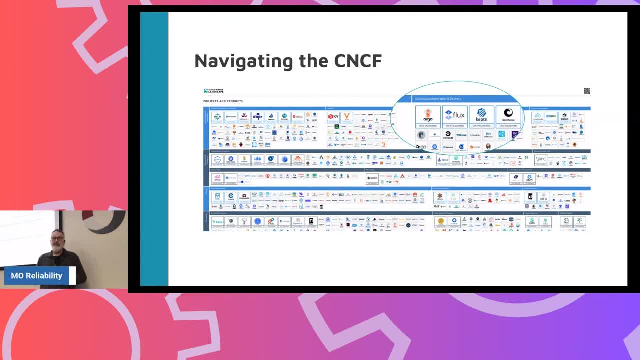 and you know, and then maybe find some, get some swag from those particular projects too. Everybody likes swag, But yeah, So no, but that's yeah, it's one of those things I don't know. 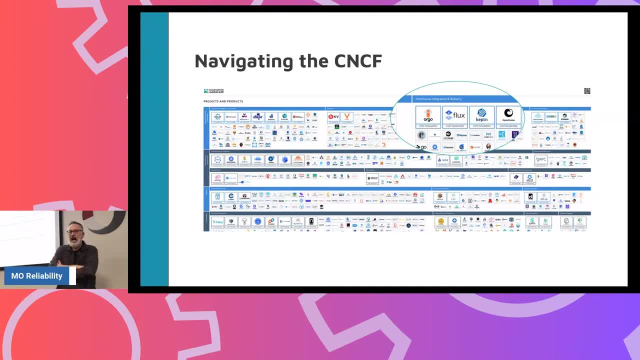 Which particular area are you thinking? I mean, I was curious about like the blue-green and the canary deployment stuff, monitoring the new feature, seeing if it's different. Yeah, One that's really interesting to me, honestly, is Kepton. 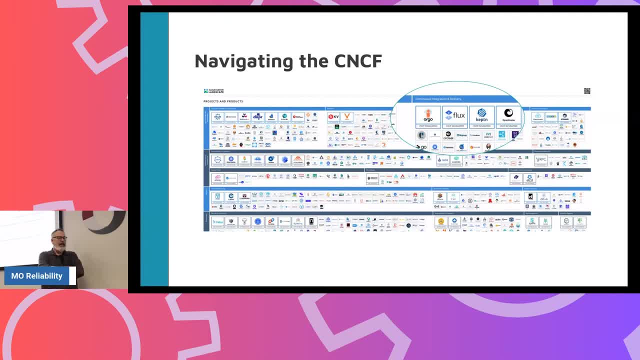 You know, but I did do a little bit of a review on that, which is: you know, I don't know, I don't know. So Kepton is was created by Dynatrace, which is really big in the observability space, right. 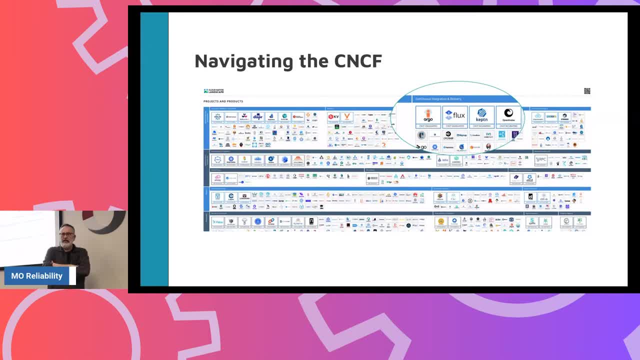 But- and in fact their engineers are really pretty much the only ones that have been really predominantly working on it, But they went through a complete rewrite. It's pretty crazy because originally I was going to do for the Kubernetes meetup. I was going, you know. 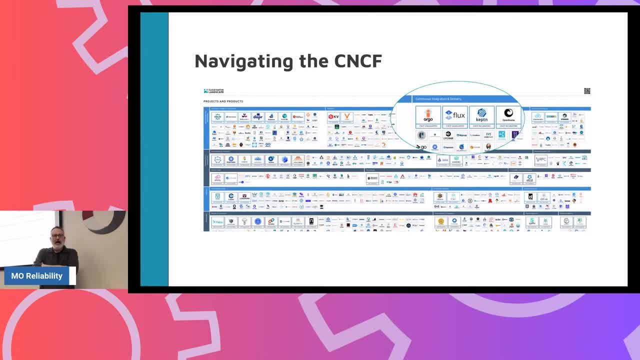 I was going to do a talk on Kepton, or well, I did it, but but my original assessment of it was from version one which had a user interface and everything and it looked really cool. I mean, it had, you know, blue or blue. 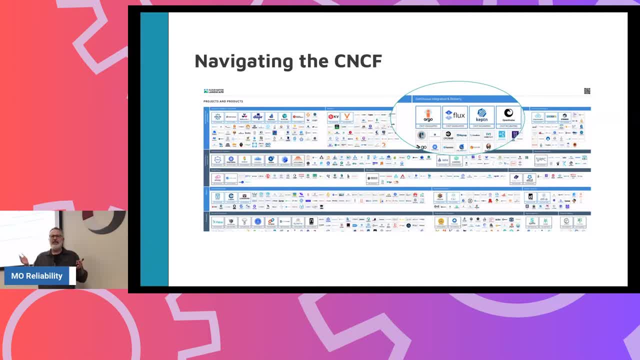 It had red and green, just like you know. you would think from like a JUnit test or something and you would see those on there and it was for each deployment, and then it would connect using a metrics adapter to you know. 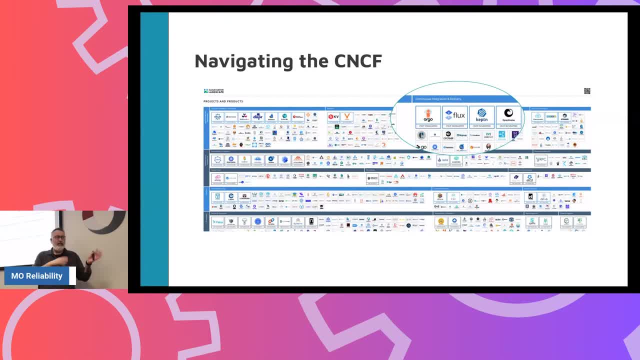 Prometheus or you know you could use Thanos or Influx data or whatever, and then it would read from those and then it would check the metrics that as the deployment was going through, So it would handle actually your Canary deployment. 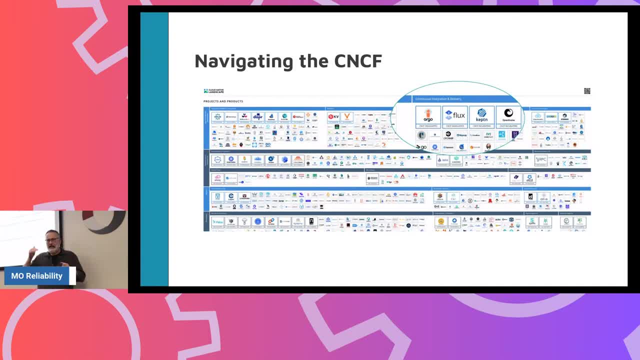 and it was watching the metrics And then it could automatically then stop a deployment and roll back even so, which was really cool, right, But it was working. but then they decided that wasn't cloud native. It wasn't cloud native enough, okay. 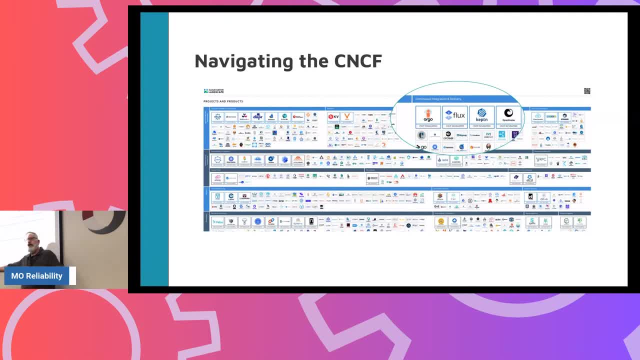 So they're like: okay, we're redoing it the entire project. So now it's completely different. Now they use the- I think it's Keptin- lifecycle management, It's something, but it's a Kubernetes custom resource. now. 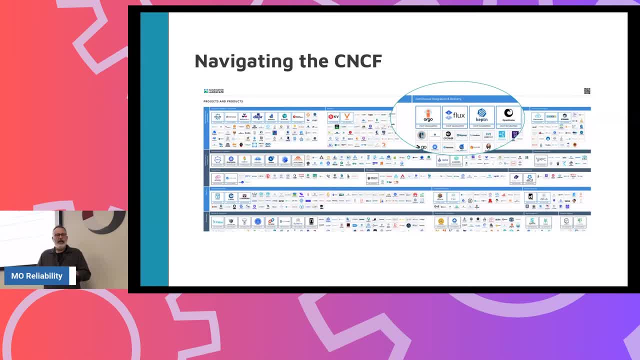 which you'll use that way. And then what's funny too is that I was talking to some of the committers on it at KubeCon and then I was kind of like I was really surprised because one of the things that they did was they got rid. 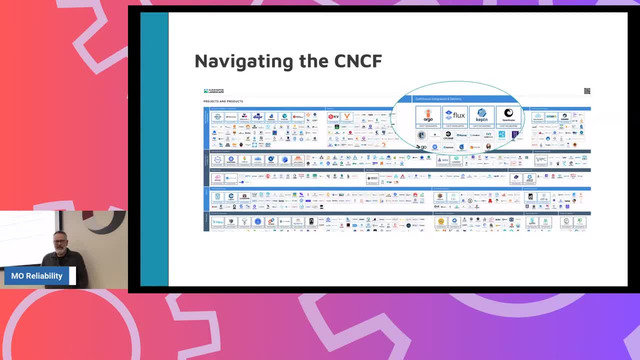 of their user interface. Now they use Grafana. So Grafana is now that dashboard view of where the deployment is. you know how many failures, how many rollbacks and things like that, But the functionality is still kind of there. 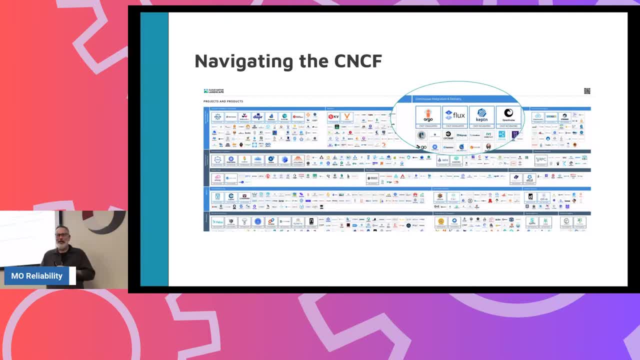 but it was a complete re-architecting and rewriting the application. So You know, in my rating scale I think I gave it a C plus because I mean I really love the thought behind it, I really love the concept and everything. 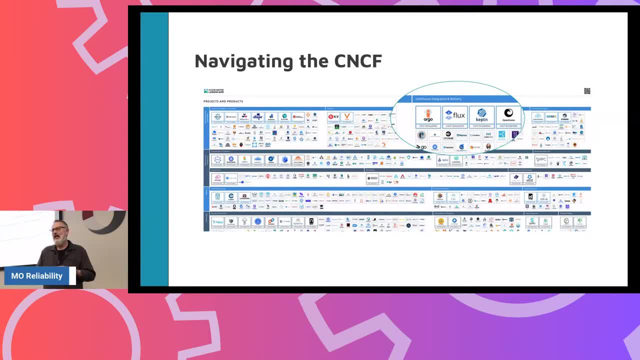 But it was just early days Now. that was almost a year ago, So I mean I haven't tried it out again since, but that was one that I really I really liked the idea on And in fact here at NISC I thought about that. 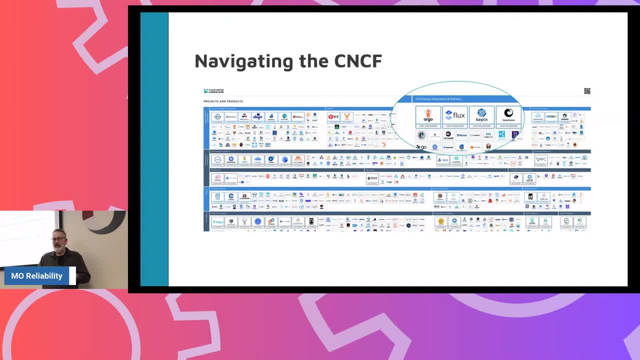 for the edge services, for deploying, you know, out to the edge. you know so. Do you compare Kepton to any of its editors, Like Argo, Yeah, no. so Argo is something that I've recently wanted to start messing around with. 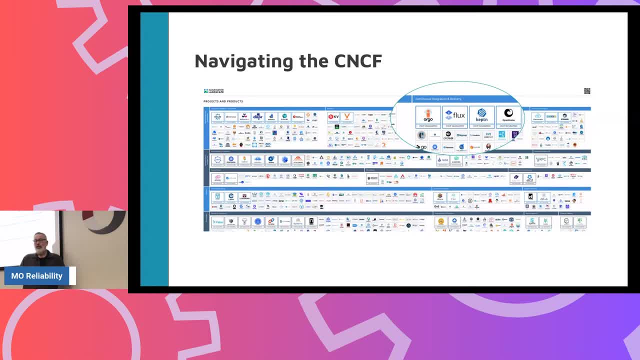 I never had before. You know, of course, Argo is the big kid on the block. That's the very popular one. It's got a lot of committers, you know. so that's Probably the one that's going to, you know. 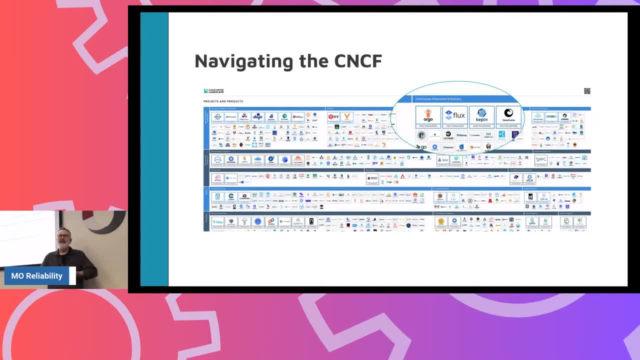 win out in the long run, And it's not really a. I wouldn't say it's well. I guess with rollouts it is a competitor, But yeah, But Argo with its under its umbrella it's got all kinds of other projects too. 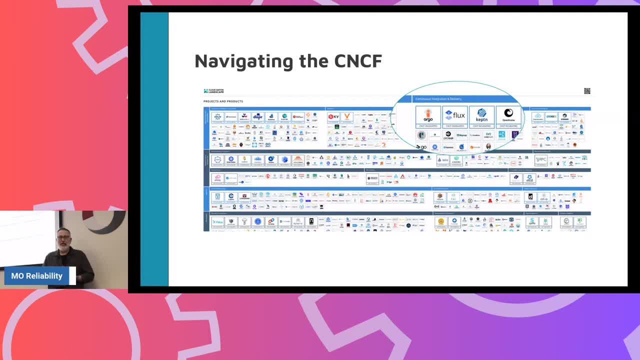 which I'm very interested in, like the workflow, Argo workflows- just for, as a controller, to be able to see the path of. you know whatever updates and where It's at in this pipeline and you know as things fork and converge. 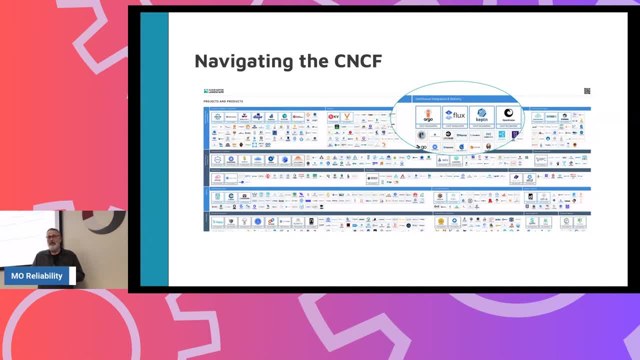 But yeah, I don't know, There's so many, like I said. I mean it's I could, literally I would love to be able to not have to work- sorry, Rob, but yeah, to be able to just go through this and go. 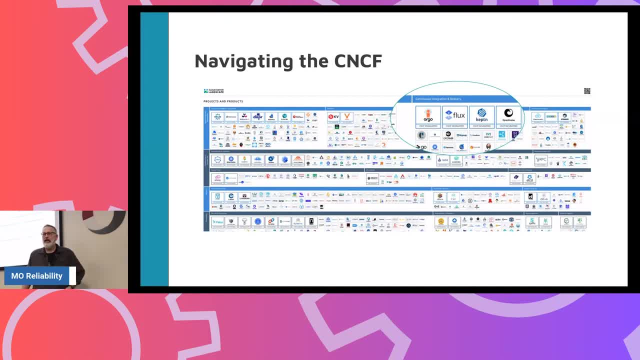 through all the different projects and then kind of do a quick evaluation. you know. But again, though I would, there's no way I would never fool myself to think that I would get in-depth knowledge on all those projects, Because there's just, it's an overwhelming landscape. 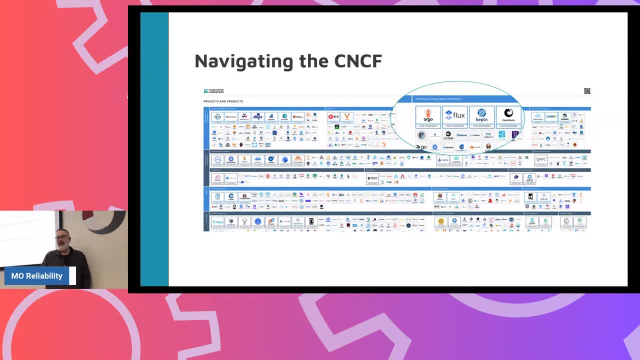 And that's just a little small section of it. I couldn't- I, you know, I couldn't fit it all on the slide. So but yeah, But no, no, I'm trying to think of some of the other ones now. 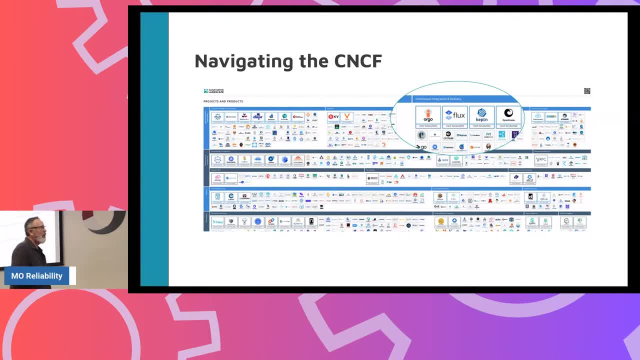 So DAP, DAPR is one that I'm pretty interested in. So that is kind of an application skeleton framework type thing with resiliency in mind. I only know that because when I was working in K6, I kind of worked with a little bit with a guy from Microsoft. 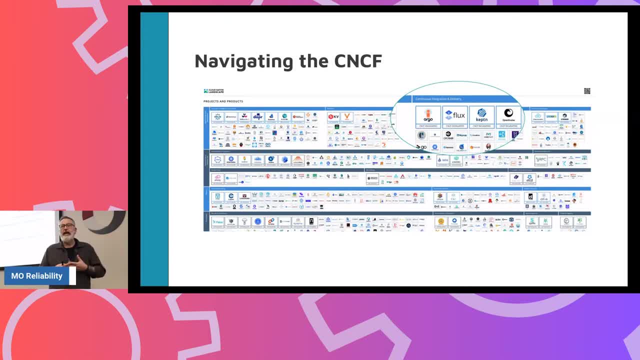 who was working on that project. In fact, he was writing tests for that using K6, the K6 operator. So he was doing some things And we were having some issues where you know the K6 operator, they inject some attributes. 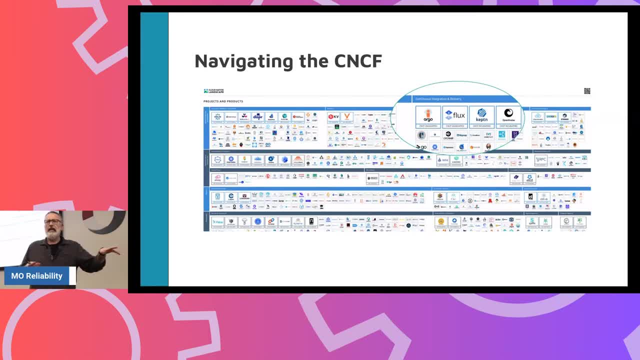 into their resource pods And I think the K6 operator was not enjoying that and would either ignore it or something. But there were some inconsistencies or incompatibilities, I should say. But that is another project though which is kind of interesting. 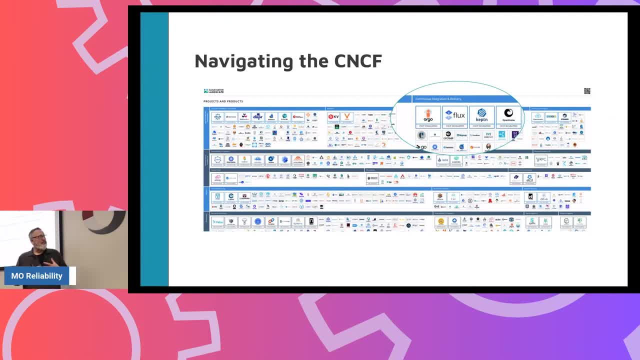 Because that's one where it's like that kind of gives you, if I'm remembering it correctly, kind of again like a base application to start from, to build off of Which you know a lot of things that are like that. 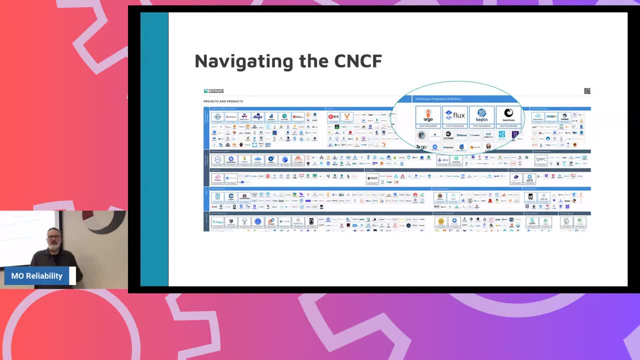 like with Spring Boot, Spring Boot has their the startspringio, where you kind of generate the skeleton. Well, I think that's that use of these libraries and that you could maybe say is equivalent to that. So is it an adapter or a language specific? 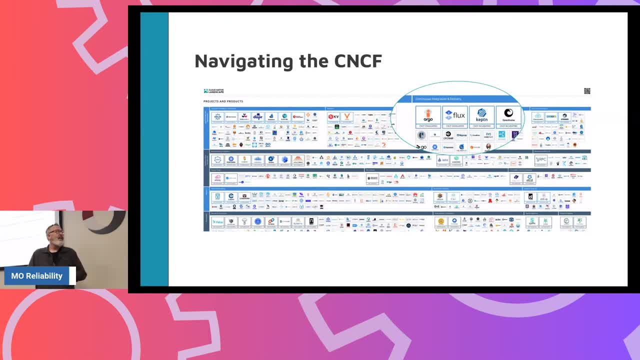 or does it have to be like it's well, it's going to be related to your Kubernetes deployments and that, So it's going to be related to that. But you know, it's as all things perform and it's written in Go. 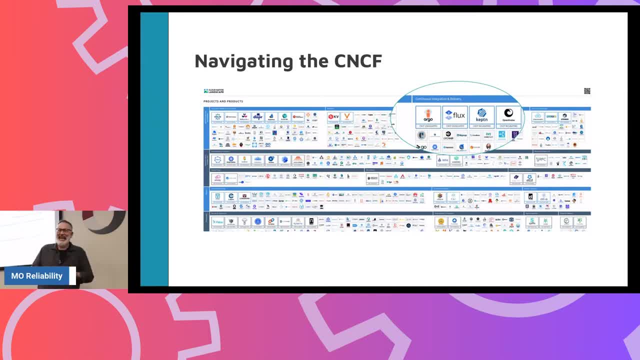 Sorry, I had to throw that in. It's expected, But yeah, no, But that is one that definitely I suggest to check into Because, again, that makes it a little bit easier on the developers to ensure that they're. 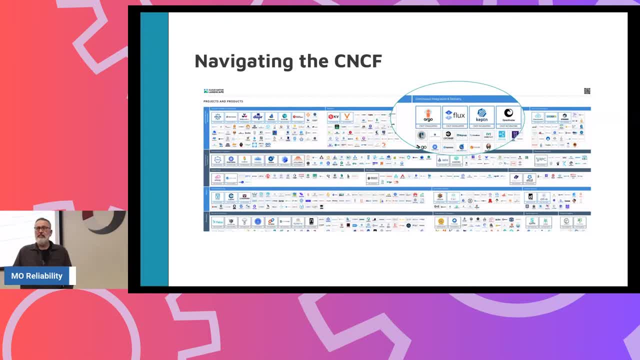 software is going to be a bit more resilient. You know which testing will prove that out as well. What was some other ones? Crossplane. Crossplane is one that's really getting popular. I don't know So very much like a Terraform. 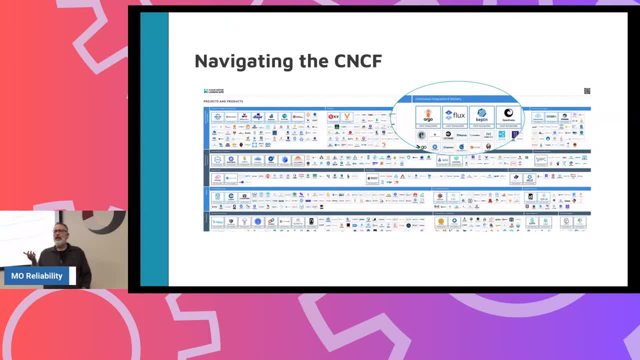 in that it's going to handle build out of infrastructure and things like that, But it's all Kubernetes based, So you would create a lot of your. instead of Terraform, you'd use Kubernetes, resources, Custom resources for the providers and things like that. 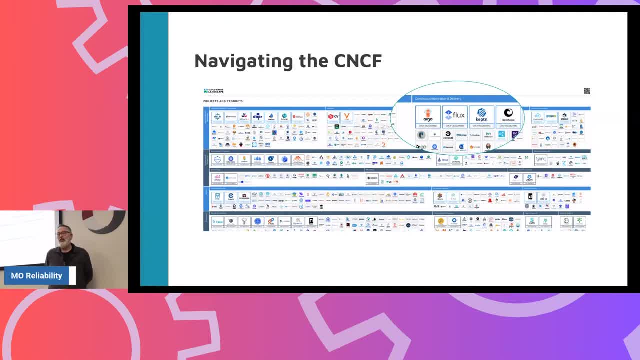 So it's somewhat, I don't know. it may be a little bit more overly complex, But it is one that is actually gaining a lot of traction. But again, how do you test that? you know those things. That's the tough part with the infrastructure as code, right? 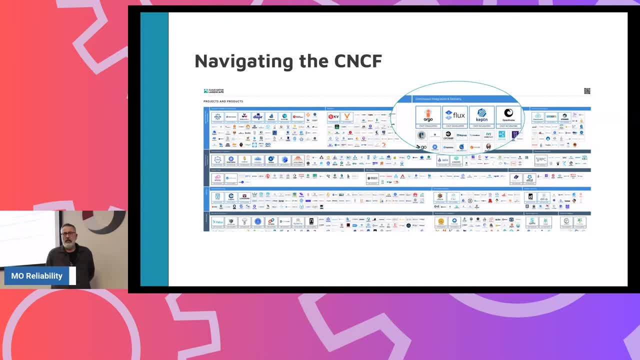 is testing. I mean, you know there's TerraTest. I've never actually tried it. I'd be curious if anybody here has actually tried it. But yeah, that's one. I don't know Because that's tough. 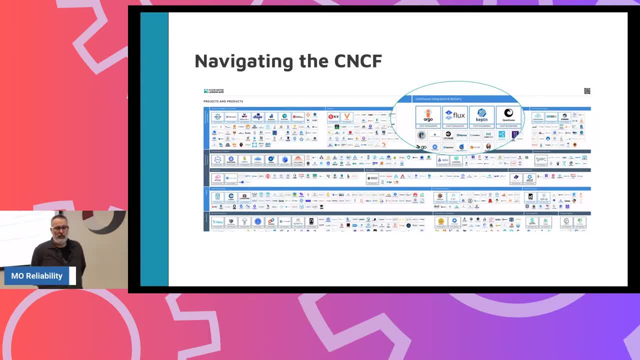 You know, and then, especially when you're trying to write things for multiple different cloud providers and such, Let's see, You know, and then of course, I'm always going to push for open telemetry. You know, everybody should be using that. 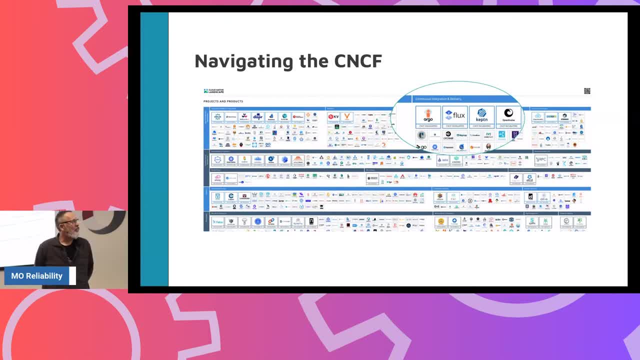 Prometheus as well. You know whether you go with Mimir or any of the other- Grafana Stack, you know, whatever. But yeah, Oh, TraceTest. I know I did a talk on that And I know folks here have tried it out. 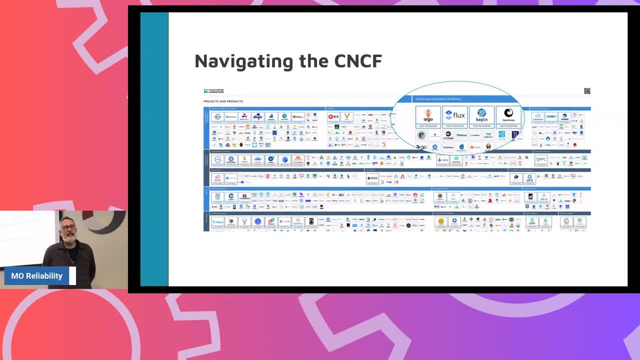 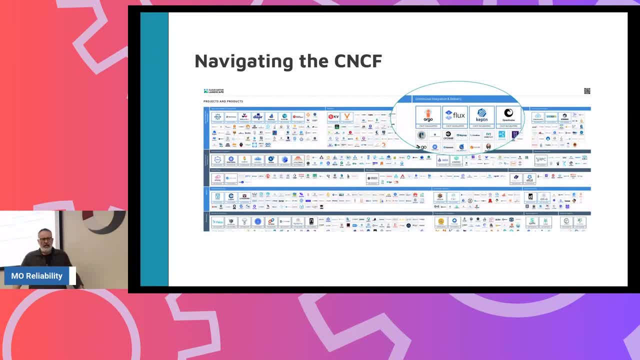 where you can do well. you can trace the activity using the open telemetry data all through an entire system and then put checks at each of the you know points, Like you know how long does it take for a message to get picked up from you know a subscriber you know. 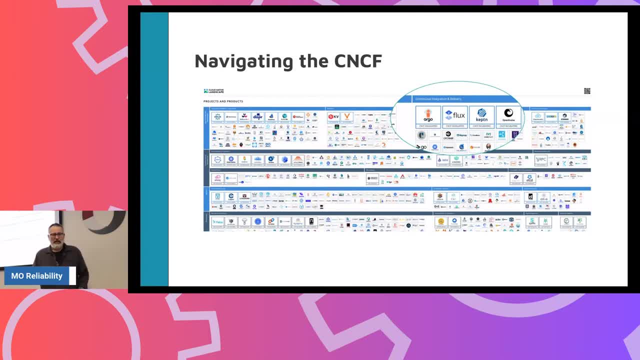 against a rabbit queue, that type of a thing. So it makes me a little nervous with the level of coupling back in the patient. Yeah, And always like how tightly are we going to create tests that only work with this exact setup? 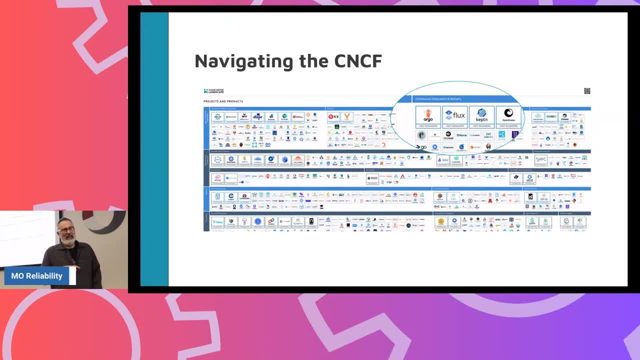 And then you change from microservice to 300 tests. That, yeah, I mean, it's a possibility. I like the idea, Yeah, But the window of what you're testing is nervous. Yeah, I agree. Yeah, With the TraceTest you can actually make something. 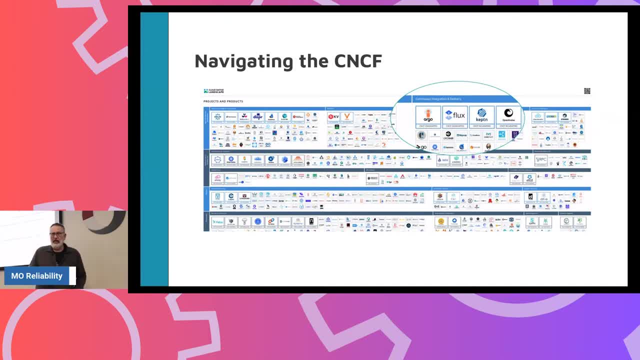 very specific to that scenario. And then, yeah, you try to go change it, while you're breaking the test immediately. you know- And unfortunately I've had a lot of code that's been like that too- where it's like: 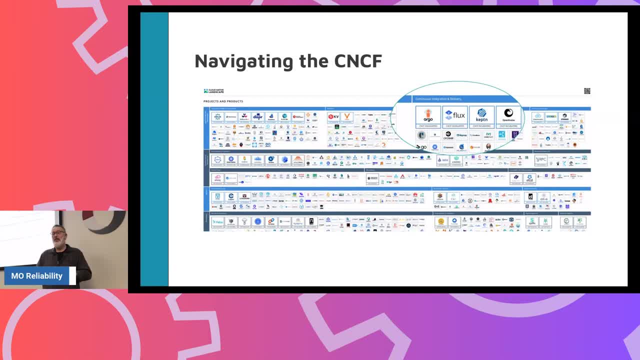 basically, your unit test is testing that your code didn't get changed. It's not checking what's coming in and out as it should. It's checking the implementation details. You know it's like: oh yeah, did it try to do this three times? 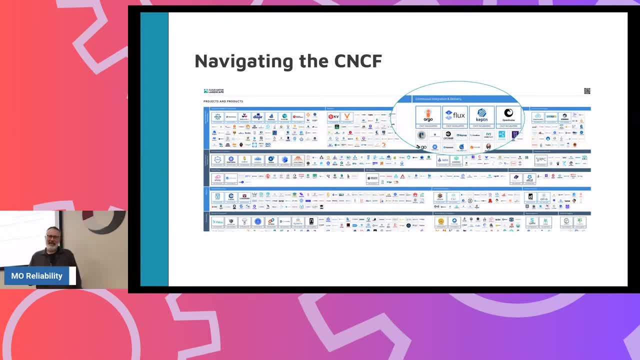 Yes, That's yeah. that doesn't matter to the test. The test should only care about. it should be like a Schrodinger's box, right, It only cares about what goes in and what comes out. Whatever happens inside, that is of no concern. 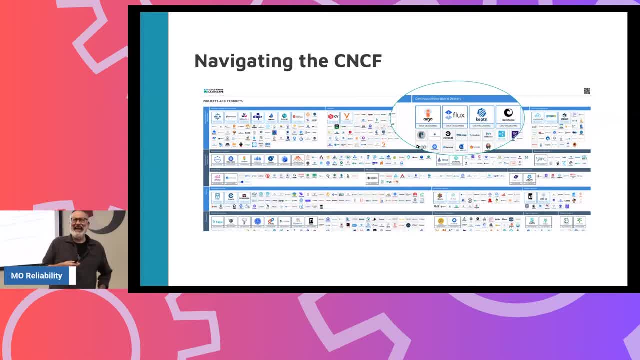 I mean, some people can type really fast and they just replace all their tests every time they're changing. Yeah, But yeah, And then let's see What other ones You know. Yeah, Of course, I will always say K6.. 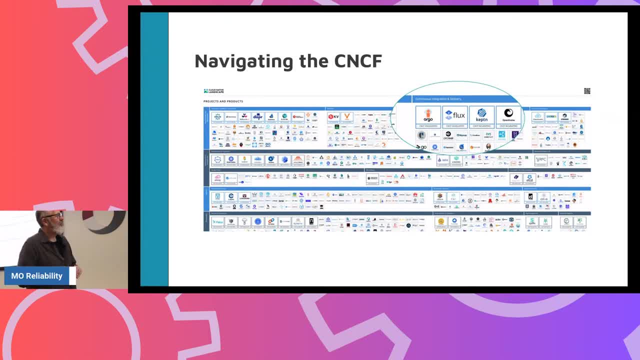 It is a product I truly believe in. Let's see. And there's some of the other big ones. I'm drawing a blank. actually, There was a question about PDPF. Yes, I think we looked at that. I'm not sure I understood what it was. 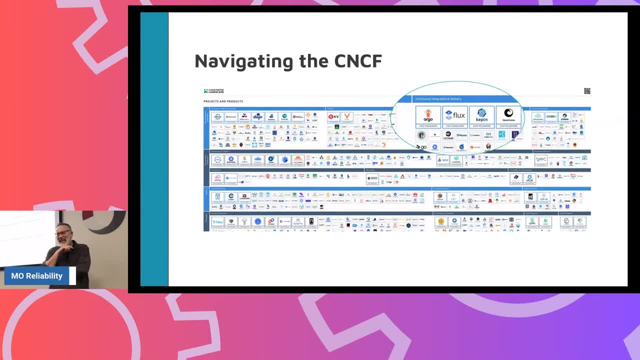 There's a little bit of magic, But yeah, I mean that way. then you can get some basic metrics without having to actually have a library directly in your code. It's just like with, if you're familiar with Java, Agent. 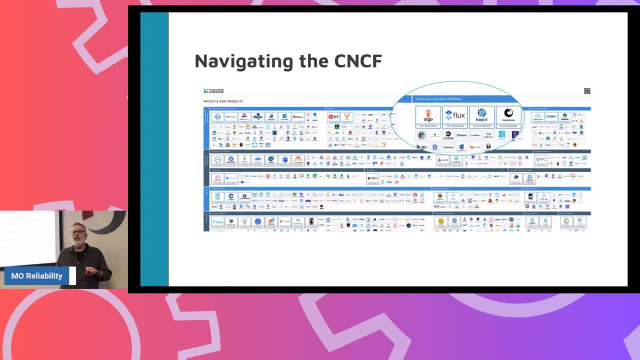 You know, Java Agent is kind of: it's not in your code but it's sitting there, Everything's going through it. Well, with eBPF, it's simply looking at the kernel, The Linux kernel, And then it's able to. I don't know how it determines messages and that. 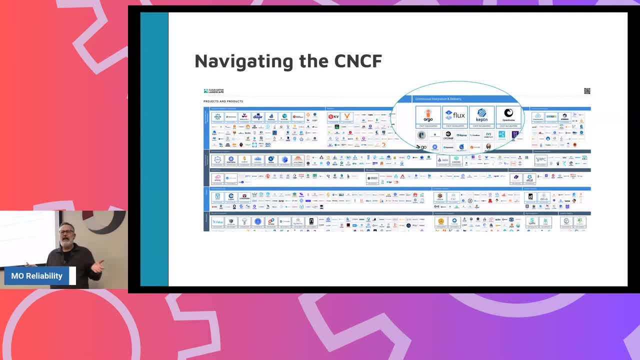 I don't know if it's just like I don't know it's recognizing patterns or there's like message headers or something is basically what it is- that go through the kernel. But yeah, So that way, then it can give you some basic metrics at least. 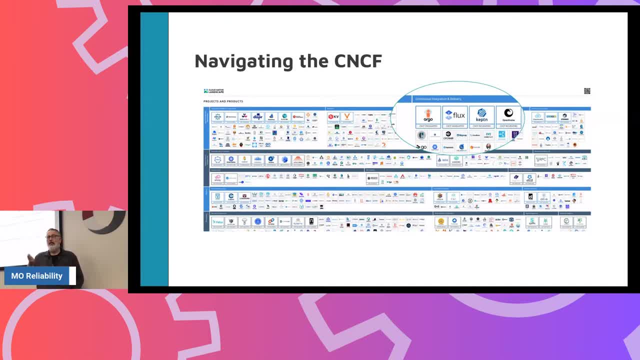 where you don't have any, But you should always still have it in your code. And one more: I know we started collecting a lot of things. Yeah, I think we got traces. I think we might even have eBPF right. 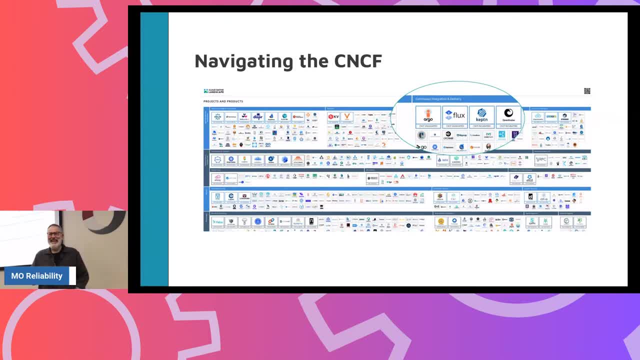 I think we turned it back on. Is there a second layer of tooling that can make it useful? You mean to actually be able to use it? Yeah, Yeah, It's like when you're filling I don't know, Can't get a good. 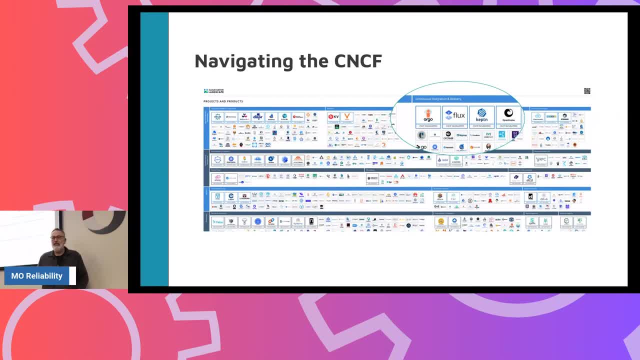 And now There's a lot of data when you're doing traces and that Yeah. But of course, Jaeger, you know, open zipkin is something tempo. There's a lot of them that use that same type of a method. 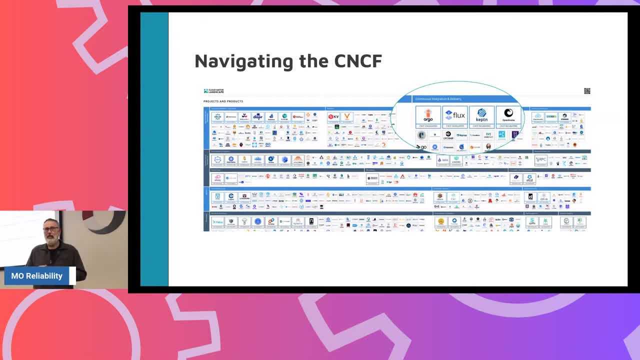 But traces you should really probably not keep around for too awful long, You know, maybe keep two weeks at the most, You know. and then also, based on that same trace data, you know, something huge to use is the continuous profile. 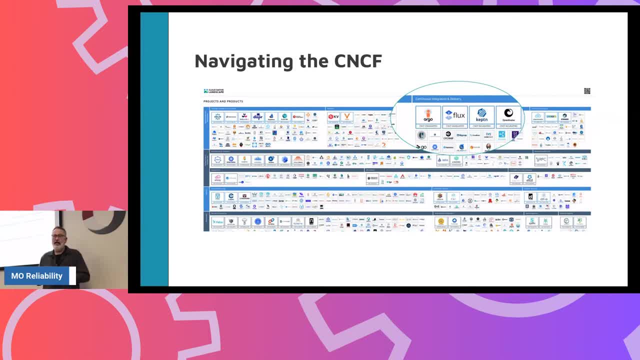 Which I know. we've kind of had some experiments going on there with PyroScope, Which that is. that's a huge thing too. The flame graphs- That's nothing cooler than flame graphs. They're isomere graphs, sir, They're not upwards okay. 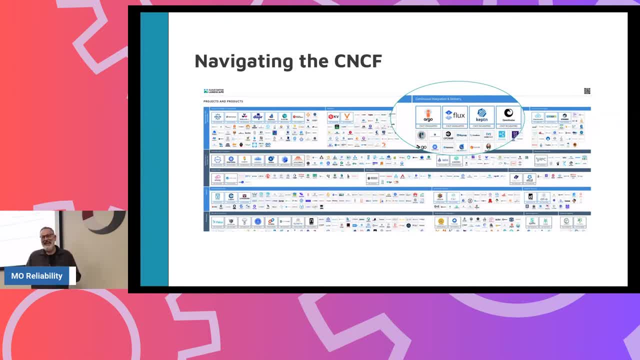 They have to be different. Yeah, yeah, I want to upload a graph that needs to be in flame: Stalagmite, stalagmite, Stalagmite, Stalagmite, whatever. Oops, Yeah, But that's that's. continuous profiling is definitely that's. that's one that I did mention. 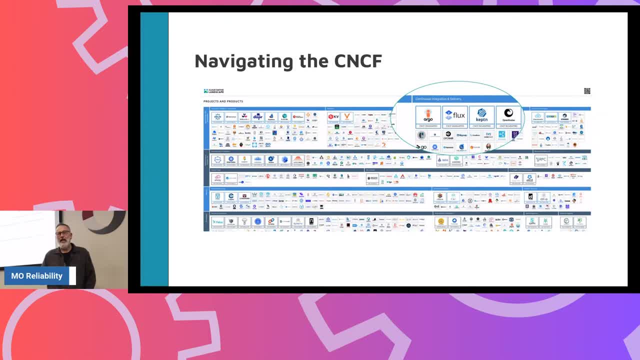 That's definitely something that needs to be in there in your process somewhere. That's that's always the thing, right? Yeah, impact the potential to impact your application. Can you get something out of it? No, Your profiling shows that you're monitoring 80% of your CPU. 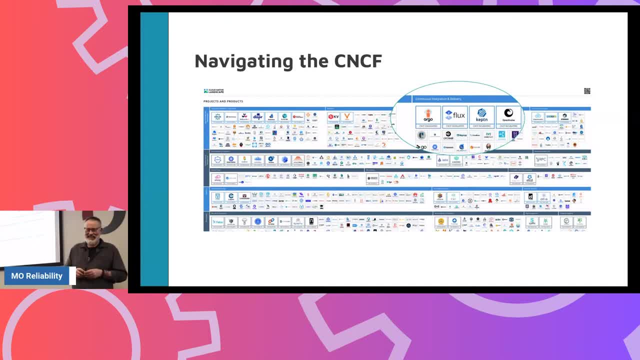 That's yeah. That's definitely not good. Yeah, Yeah. And I know one of the things that I always liked Was the service mesh. I enjoyed it, enjoyed that Linkerd a while back, but we had some issues, I think, with some of the SSL. 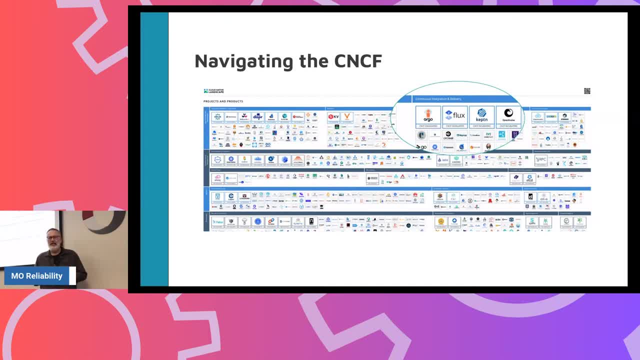 But yeah, I don't even remember what that was, but that was years ago. so, Male Speaker: 6 Male Speaker, 7 Male Speaker, 8 Male Speaker, 9 Male Speaker, 10 Male Speaker, 11 Male Speaker, 12 Male Speaker- 13. 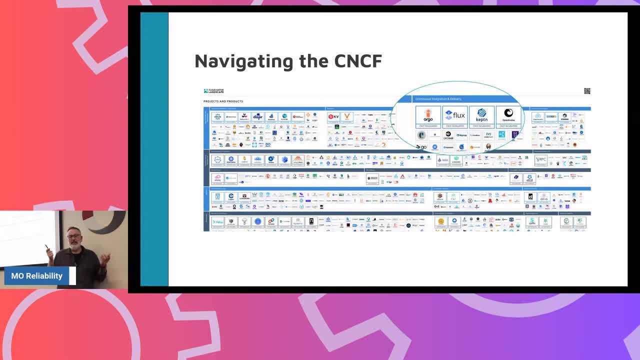 Male Speaker: 14 Male Speaker, 15 Male Speaker, 16 Male Speaker, 17 Male Speaker, 18 Male Speaker, 19 Male Speaker, 20 Male Speaker, 21 Male Speaker, 22 Male Speaker, 23 Male Speaker, 24 Male Speaker, 25 Male Speaker, 26. 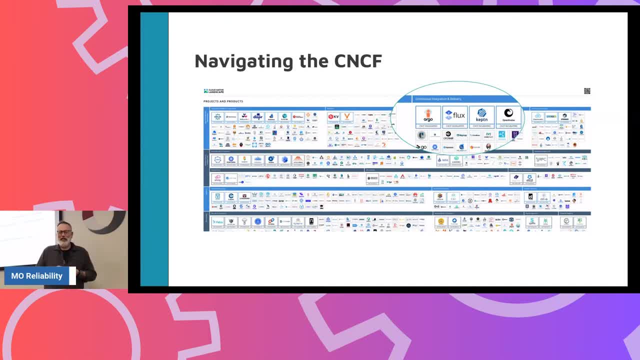 Male Speaker: 27 Male Speaker, 29 Male Speaker, 30 Male Speaker, 31 Male Speaker, 32 Male Speaker, 33 Male Speaker, 34 Male Speaker, 35 Male Speaker, 36 Male Speaker, 37 Male Speaker, 39 Male Speaker, 40 Male Speaker 41. 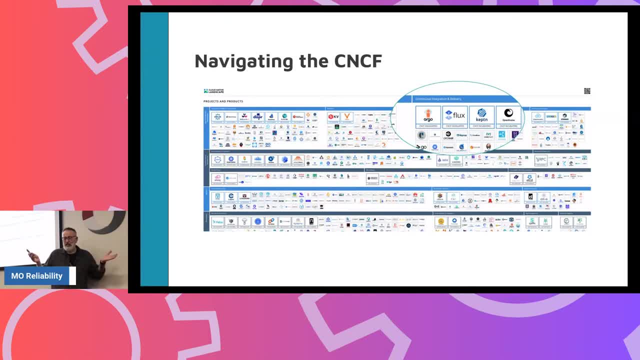 Male Speaker, 42 Male Speaker, 43 Male Speaker, 44 Male Speaker, 45 Male Speaker, 46 Male Speaker, 47 Male Speaker, 48 Male Speaker, 49 Male Speaker, 50 Male Speaker, 51 Male Speaker, 52 Male Speaker, 53 Male Speaker 54. 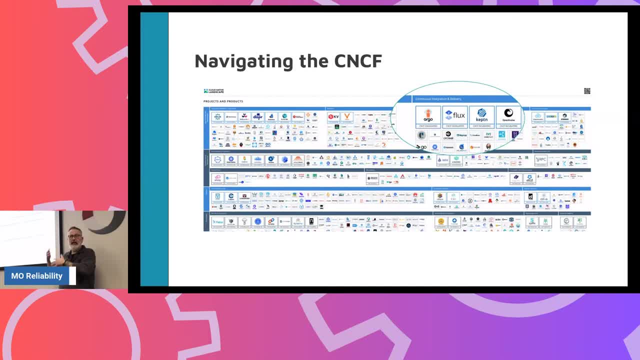 Male Speaker, 55 Male Speaker, 56 Male Speaker, 56 Male Speaker, 57 Male Speaker, 58 Male Speaker, 59 Male Speaker, 60 Male Speaker, 61 Male Speaker, 62 Male Speaker, 63 Male Speaker, 64 Male Speaker, 65 Male Speaker 67. 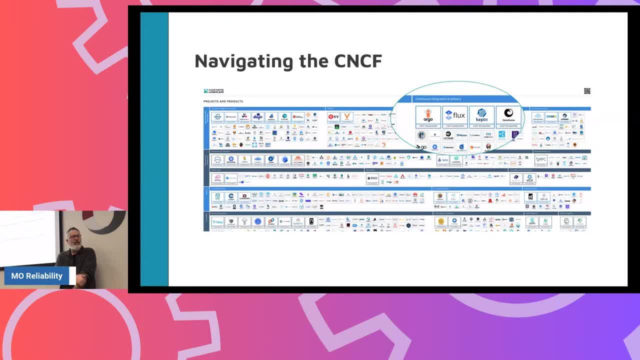 Male Speaker, 68 Male Speaker, 69 Male Speaker, 60 Male Speaker, 61 Male Speaker, 61 Male Speaker, 62 Male Speaker, 63 Male Speaker, 63 Male Speaker, 64 Male Speaker, 65 Male Speaker, 66 Male Speaker, 66 Male Speaker 67. 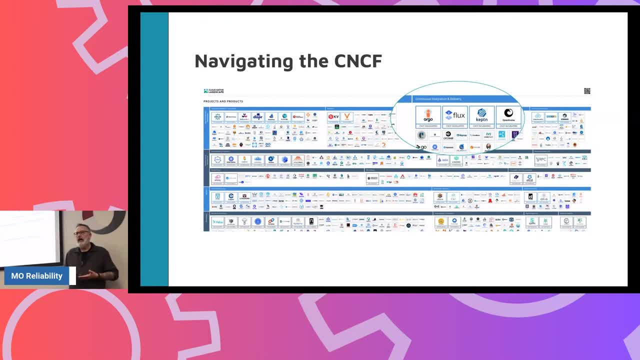 Male Speaker, 68 Male Speaker, 69 Male Speaker, 61 Male Speaker, 61 Male Speaker, 62 Male Speaker, 63 Male Speaker, 63 Male Speaker, 64 Male Speaker, 65 Male Speaker, 66 Male Speaker, 67 Male Speaker, 61 Male Speaker 61. 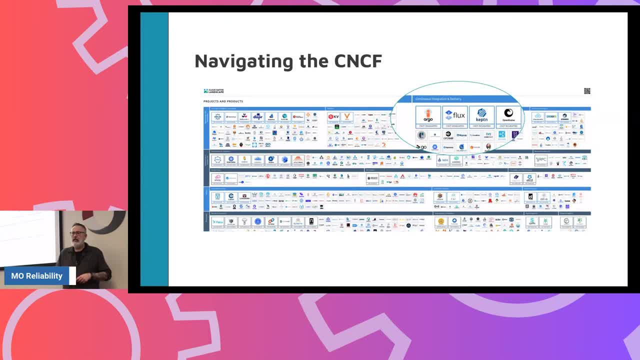 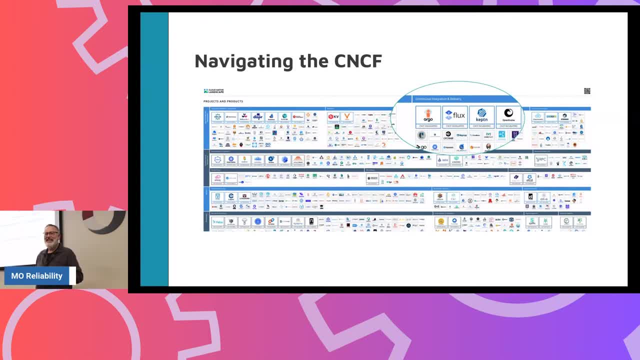 Male Speaker, 68 Male Speaker, 68 Male Speaker, 69 Male Speaker, 69 Male Speaker, 70 Male Speaker, 71 Male Speaker, 71 Male Speaker, 71 Male Speaker, 72 Male Speaker, 72 Male Speaker, 73 Male Speaker, 73 Male Speaker, 74. 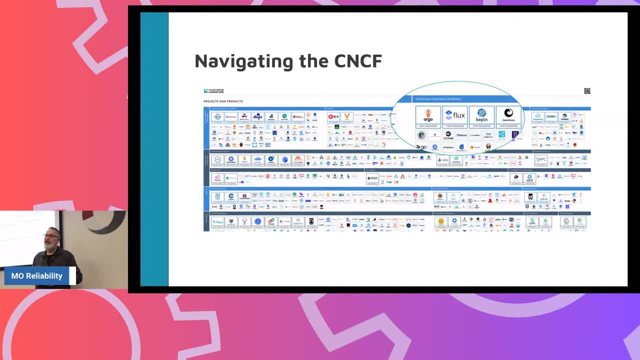 Male Speaker: 74 Male Speaker. 75 Male Speaker. 76 Male Speaker, 76 Male Speaker. 76 Male Speaker. 77 Male Speaker, 78 Male Speaker, 79 Male Speaker, 79 Male Speaker. 78 Male Speaker. 79 Male Speaker, 80 Male Speaker 71. 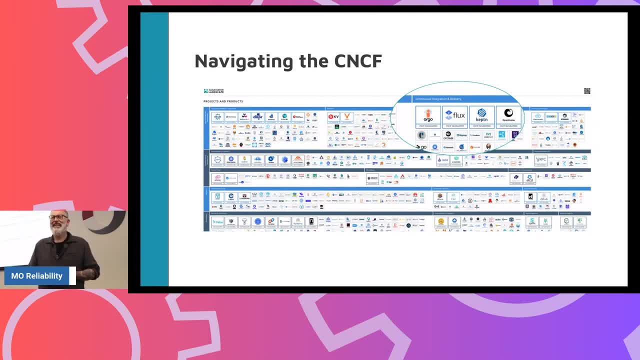 Male Speaker: 72 Male Speaker, 73 Male Speaker, 73 Male Speaker, 74 Male Speaker, 74 Male Speaker, 75 Male Speaker, 76 Male Speaker, 75 Male Speaker, 76 Male Speaker, 76 Male Speaker, 76 Male Speaker, 77 Male Speaker, 78. 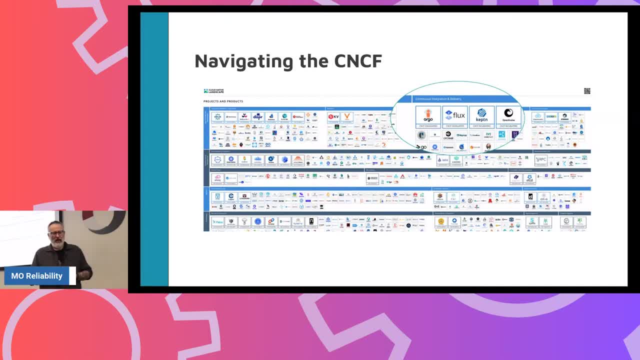 Male Speaker: 79 Male Speaker, 79 Male Speaker, 80 Male Speaker, 71 Male Speaker, 71 Male Speaker, 72 Male Speaker, 73 Male Speaker, 74 Male Speaker, 74 Male Speaker, 75 Male Speaker, 75 Male Speaker, 76 Male Speaker, 76. 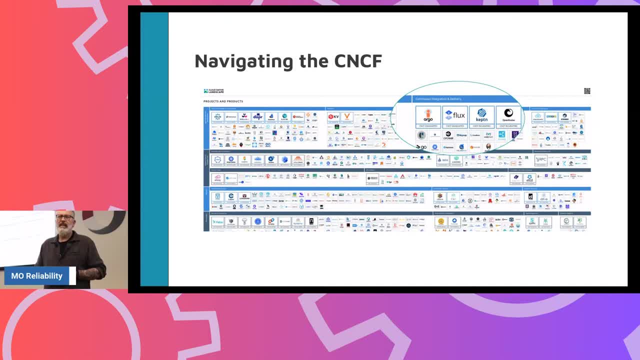 Male Speaker, 77 Male Speaker, 78 Male Speaker, 78 Male Speaker, 79 Male Speaker, 79 Male Speaker, 79 Male Speaker, 70 Male Speaker, 71 Male Speaker, 71 Male Speaker, 72 Male Speaker, 72 Male Speaker, 73 Male Speaker, 73. 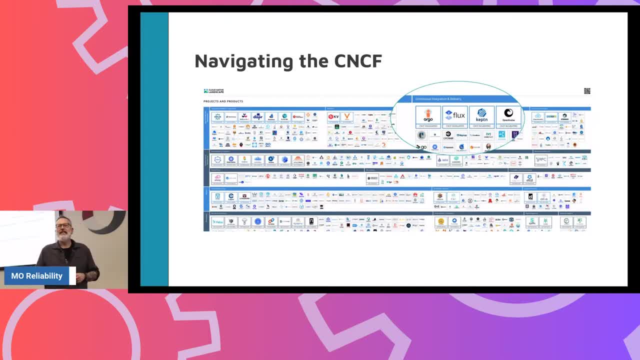 Male Speaker: 74 Male Speaker, 74 Male Speaker, 75 Male Speaker, 75 Male Speaker, 75 Male Speaker, 76 Male Speaker, 76 Male Speaker, 77 Male Speaker, 78 Male Speaker, 79 Male Speaker, 79 Male Speaker, 79 Male Speaker 70. 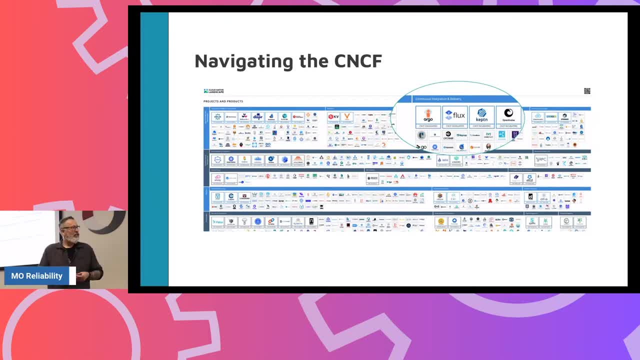 Male Speaker: 71 Male Speaker, 72 Male Speaker, 78 Male Speaker, 78 Male Speaker. 78 Male Speaker. 79 Male Speaker. 78 Male Speaker, 79 Male Speaker, 79 Male Speaker, 79 Male Speaker, 70 Male Speaker, 70 Male Speaker 71. 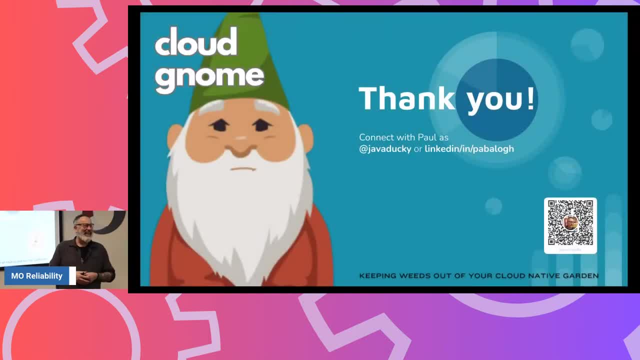 Male Speaker: 71 Male Speaker 71 Male Speaker, 72 Male Speaker, 72 Male Speaker, 73 Male Speaker. 74 Male Speaker, 74 Male Speaker, 75 Male Speaker, 74 Male Speaker. 75 Male Speaker 75.